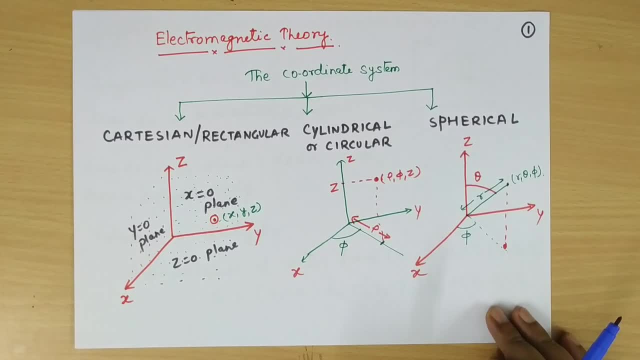 Hello friends, welcome to my YouTube channel, RF Design Basics. Now I am going to start a fresh course, which is electromagnetic theory, and in that the first topic is the coordinate system and vector convergence. So we are going to study that In general there are three types of 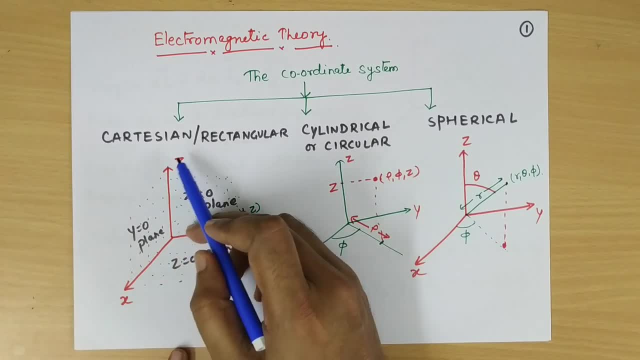 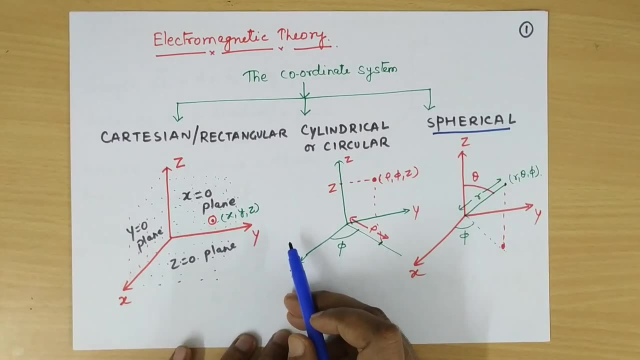 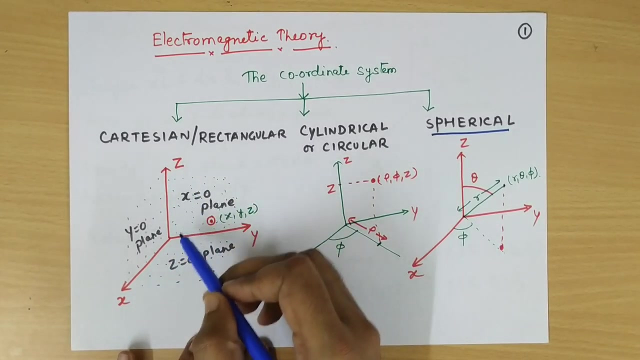 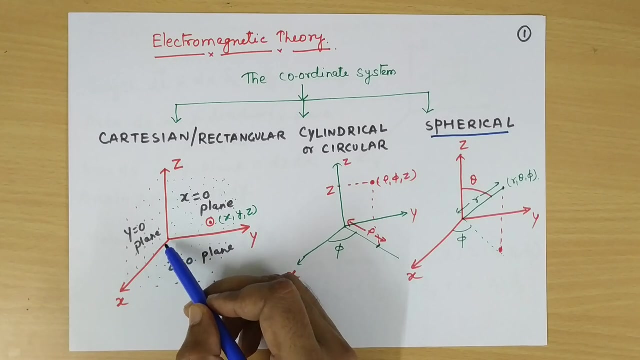 coordinate system. The first one is called rectangular coordinate system, second one is cylindrical coordinate system and third one is called a spherical coordinate system. So in rectangular coordinate system we have three axes, x, y, z, which is perpendicular to each other, and we can define any point by taking the number of units in x. 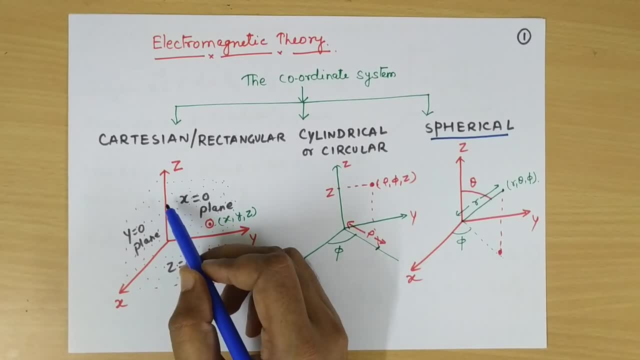 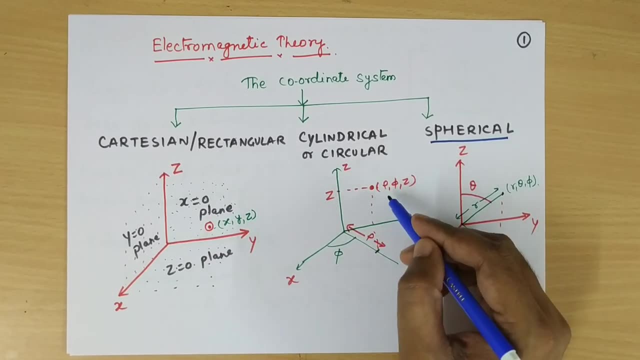 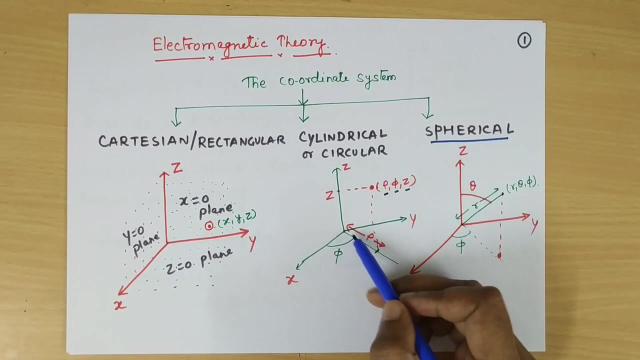 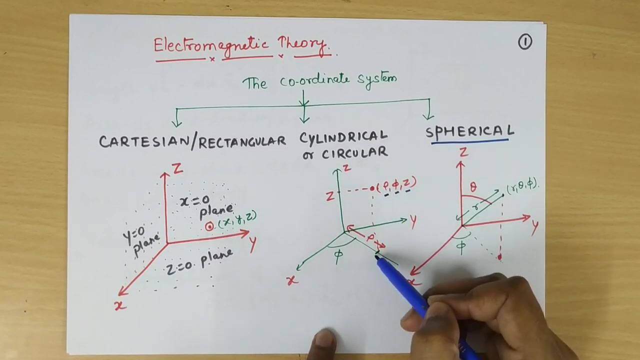 number of units in y and number of units in z direction. Similarly, in the cylindrical coordinate system we have three coordinates, which is rho, phi and z. The rho is the distance from the center to the projection of the point on x y plane. So if I have a point, 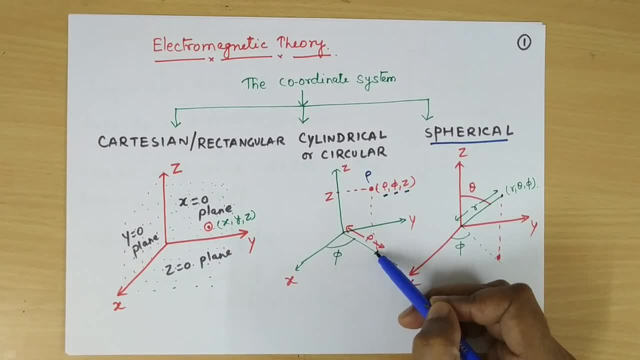 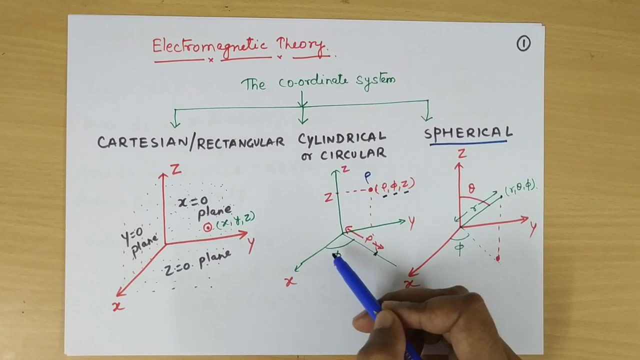 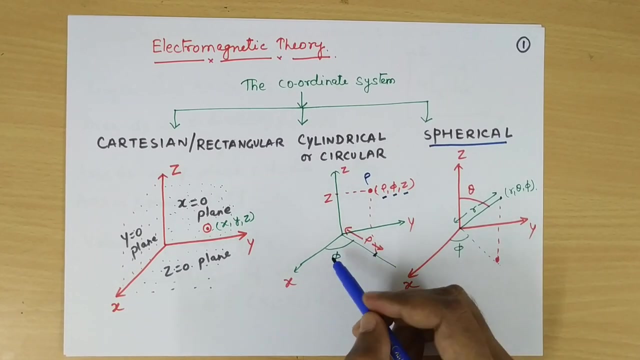 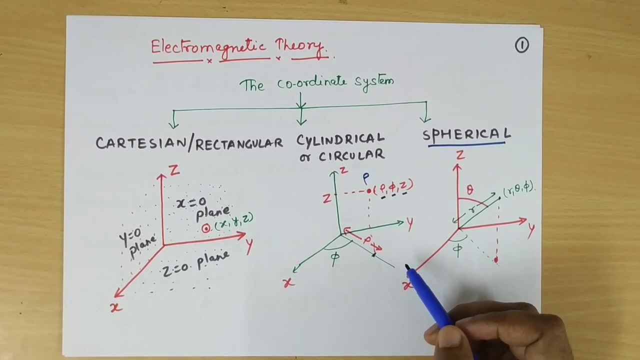 p here and I take a projection on x- y plane, then the distance from origin to this projection is rho And the angle made on x axis by this projection vector is called phi, and z is same as the rectangular coordinate system. So here we define any point as rho, phi and z. 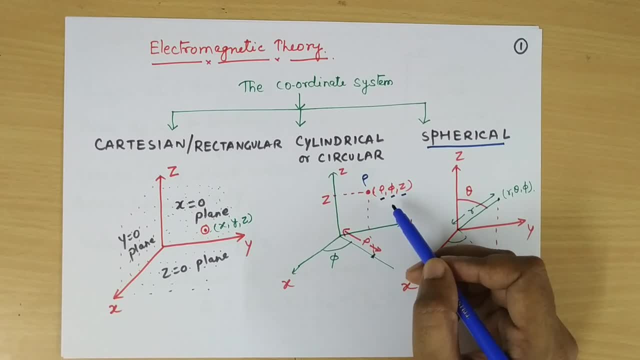 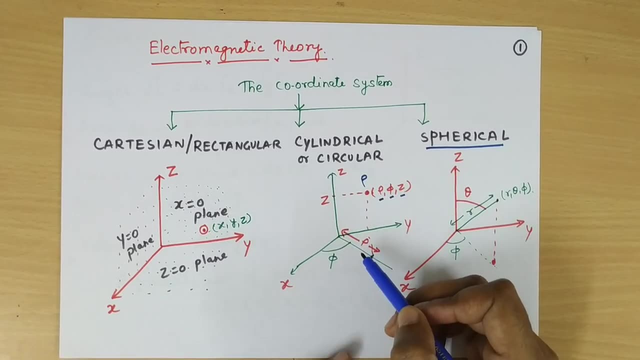 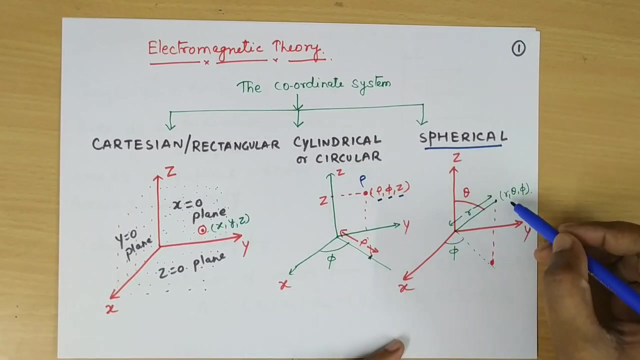 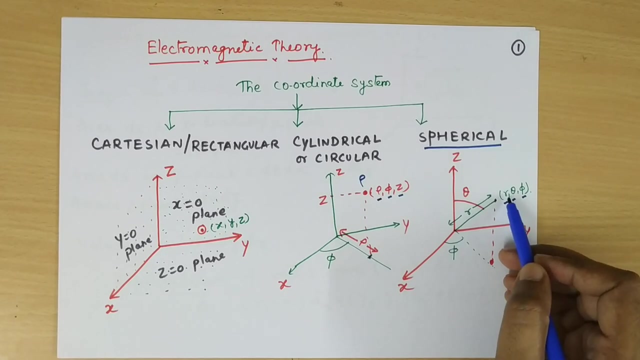 We will be learning the relation between the rectangular coordinate system and cylindrical coordinate system in our next slides. Here the spherical coordinate system is having again three coordinates: r, theta and phi, which will be perpendicular to each other in terms of its unit vector, where r is the shortest distance between origin and the given point. let's say, given point is p. 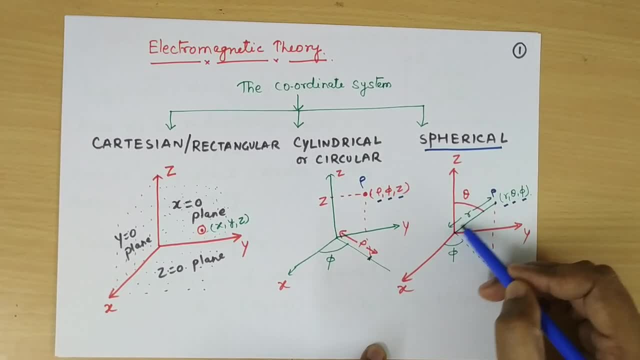 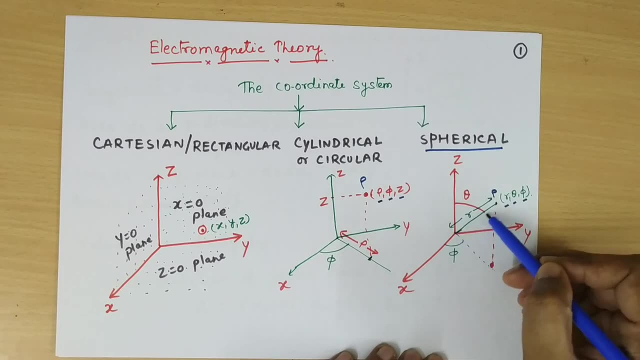 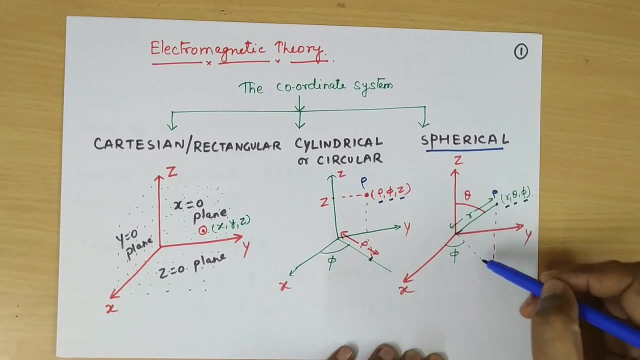 So the distance from the origin to this point is r and theta is defined as the angle made on z-axis by this vector r. So this angle is theta and phi is again similar to the cylindrical coordinate system. that means it is the projection of this point and the angle made by this projection. 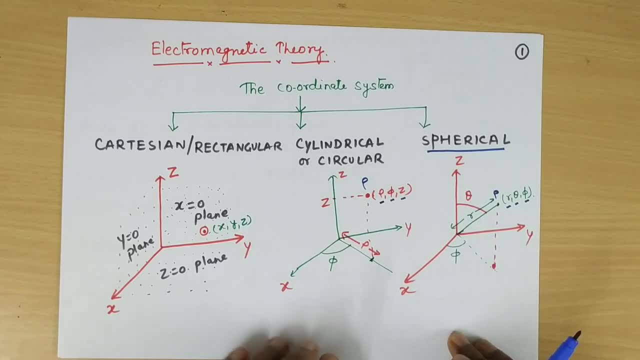 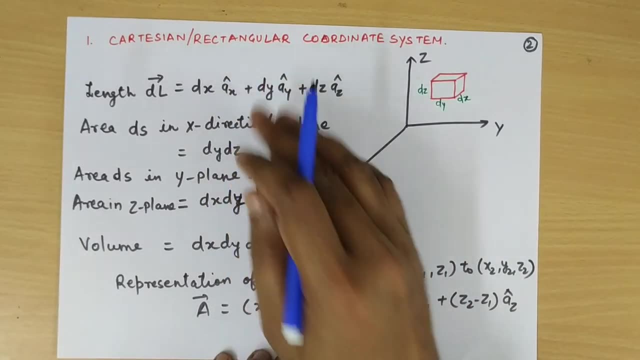 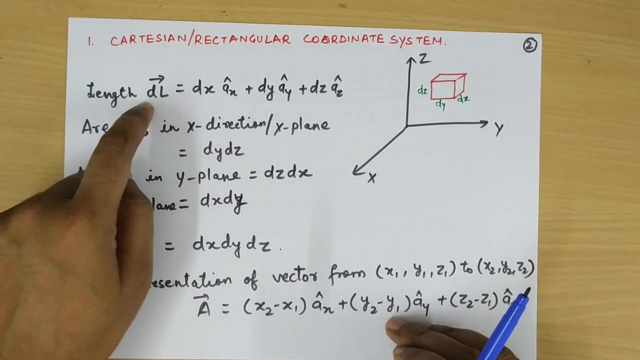 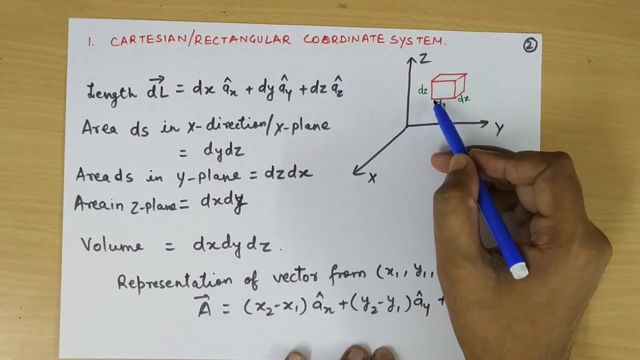 vector with r, So this x-axis is called phi. Now, first of all, we will take the Cartesian, or rectangular, coordinate system and we will try to understand how to write its length vector, or area vector, or the volume vector. For that, let us take the incremental length in each of these three coordinates, that is. 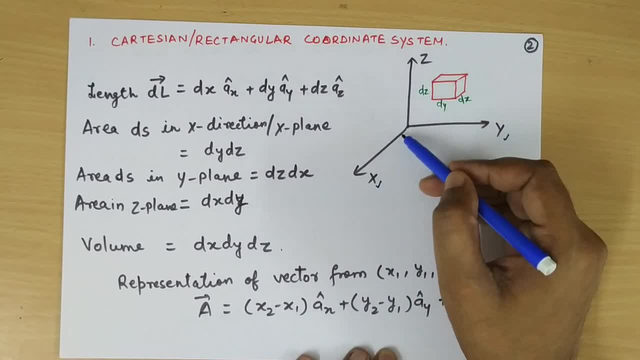 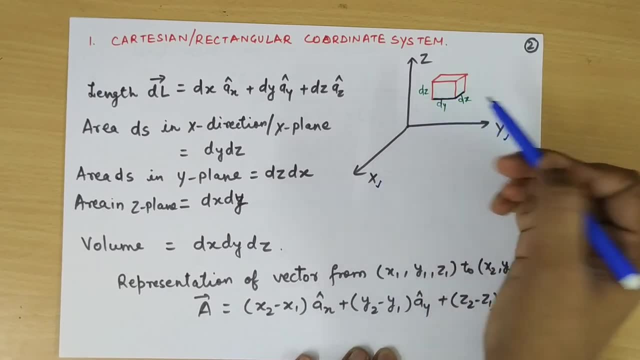 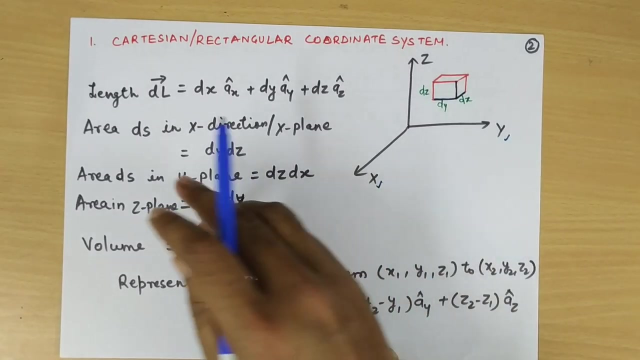 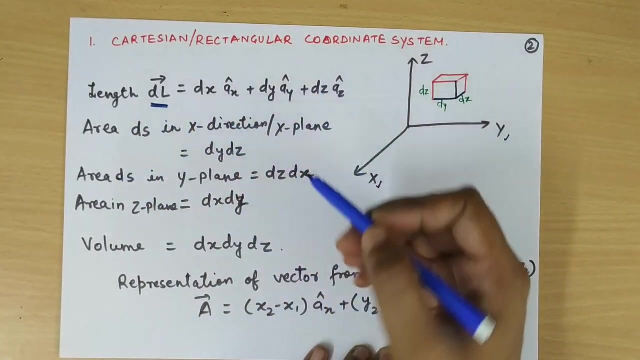 x, y and theta. So here in x direction the incremental length is dx, in y direction the incremental length is dy and in z direction the incremental length is dz. So to write the vector, length, vector dl, that is incremental length vector we have to take. 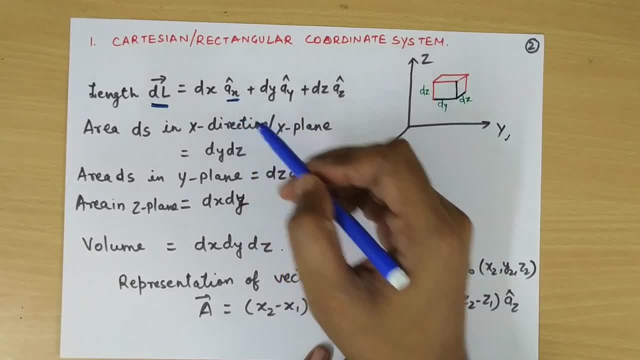 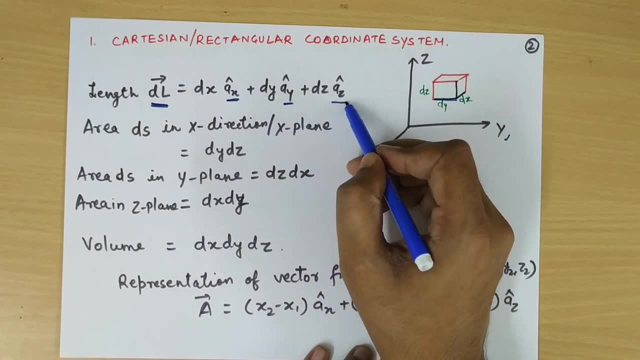 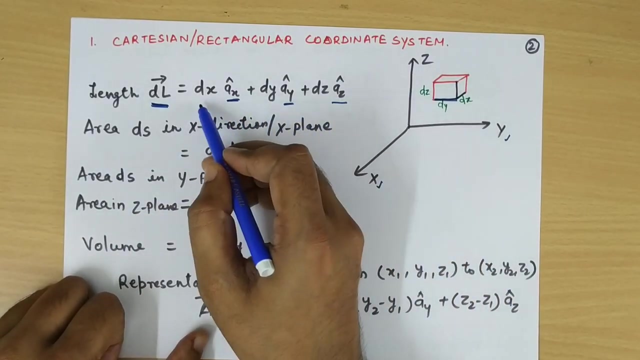 the incremental length in x and the unit vector in x direction. Similarly incremental length in y and unit vector in y direction and for z direction. So it will be dx, ax, dy, ay and dz az. So addition of these will: 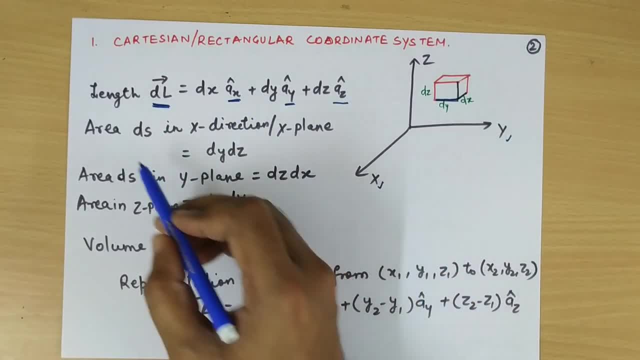 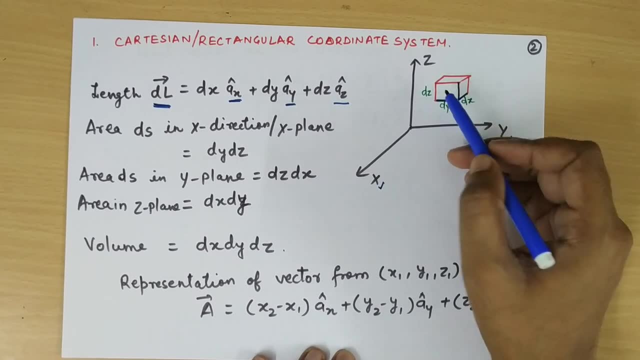 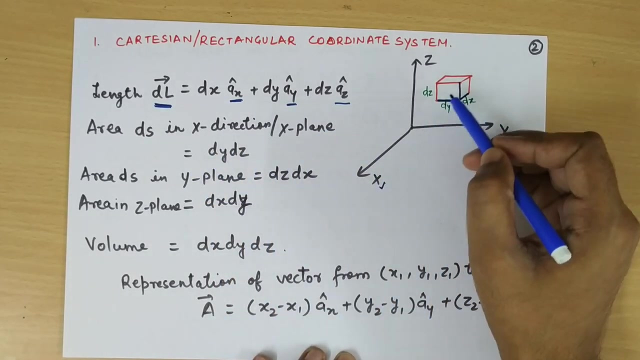 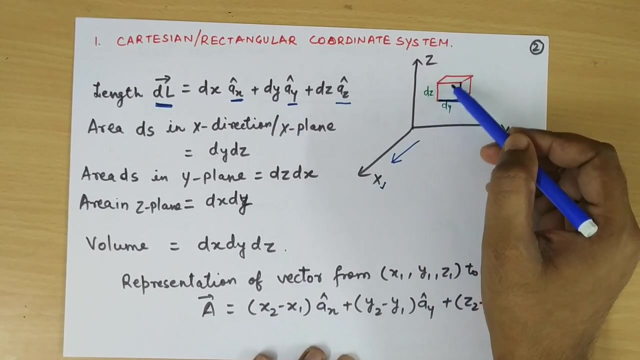 give the length vector. To find area vector in rectangular coordinate system, first of all we have to define on which plane we are finding area. Let's say we are trying to find area vector in x direction, So this is our x direction To find this area vector, the. 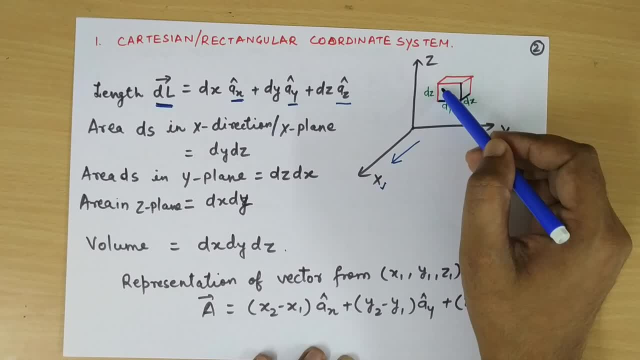 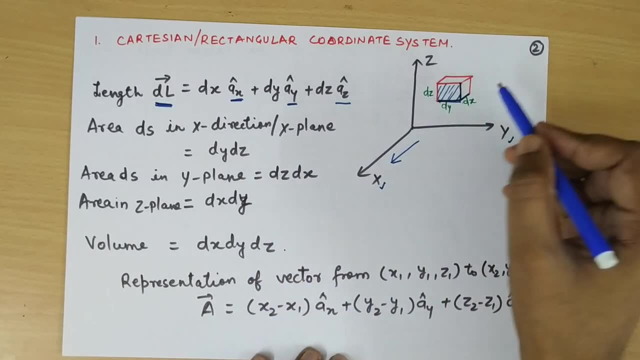 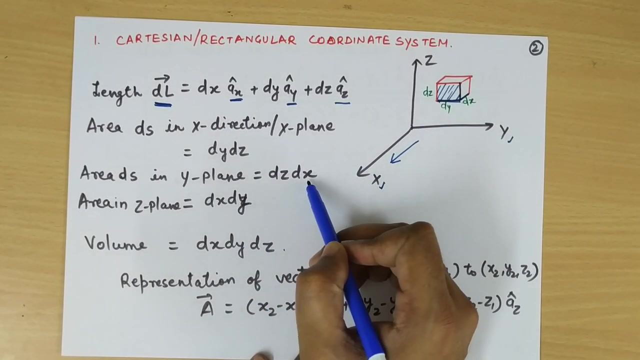 incremental length in dy and dz will be multiplied together to know the area of this, So that will be dy into dz. Similarly, if we are taking area vector in this plane, So this plane is dx multiplied by dz, So it will be dz into dx. because when 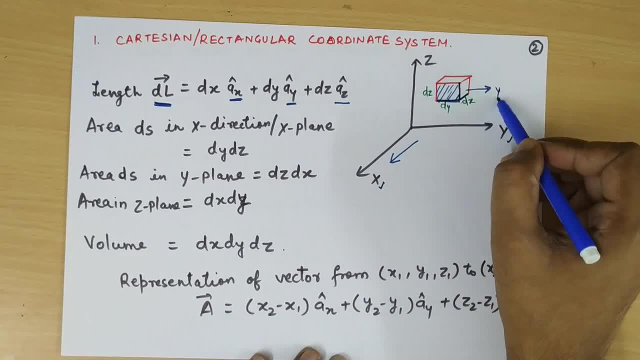 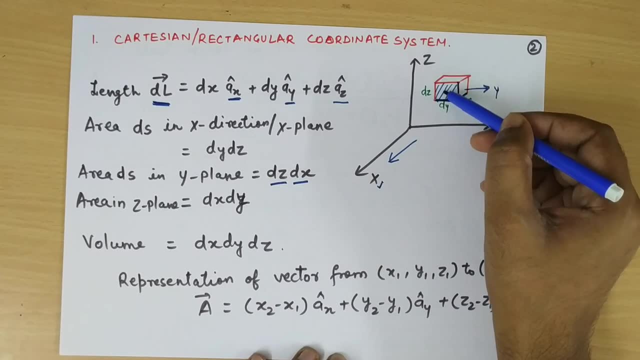 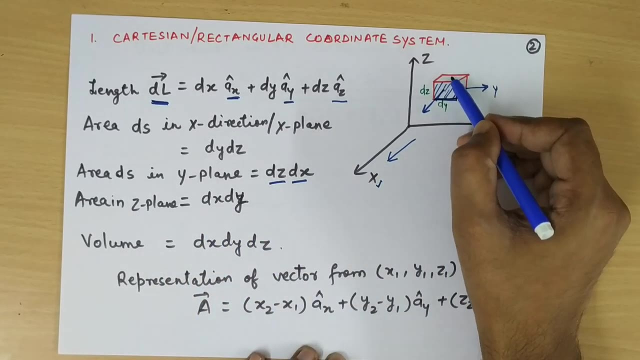 we take the area vector in y direction, this will be z into x multiplication, So we can write area vector as dz into dx. So the first area vector was this. Now this area vector is dz into dx, And in z direction, that is, in the upward direction, the area vector will be dx into dy And the 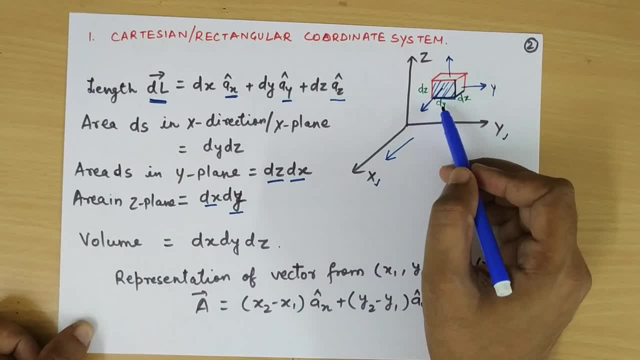 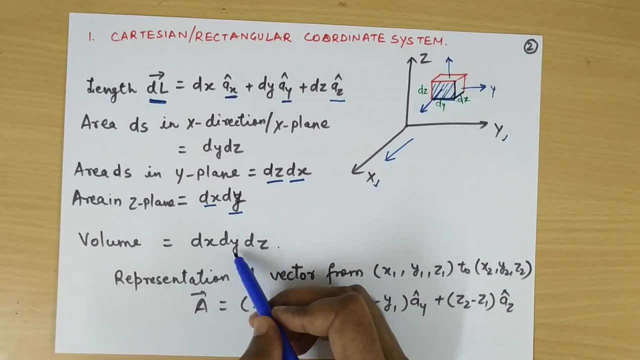 volume of this coordinate system. we can write the volume of this small unit as dx, dy into dz, which is the incremental length in x, y and z respectively. Now, to represent any vector in rectangular coordinate system which is extended from point x1, y1, z1 to x2, y2 and z2.. We simply take the difference of these. 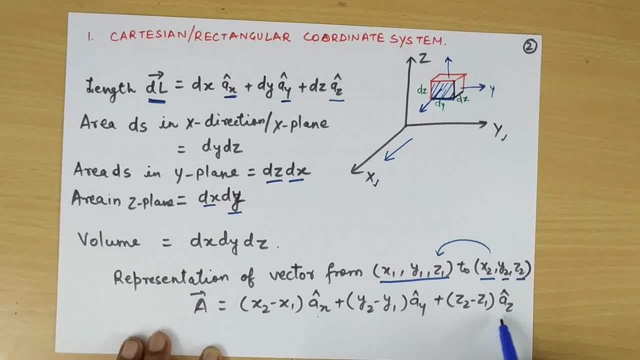 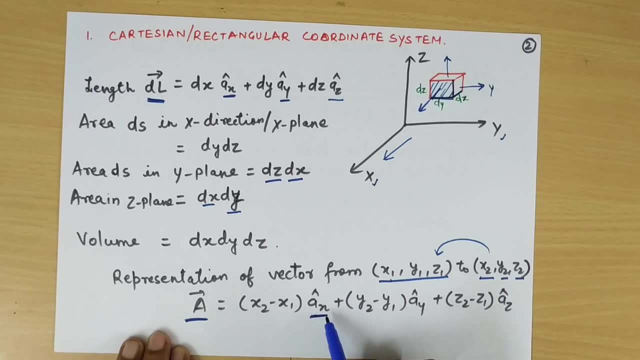 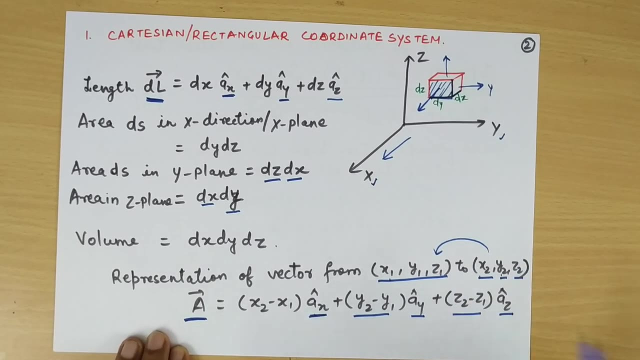 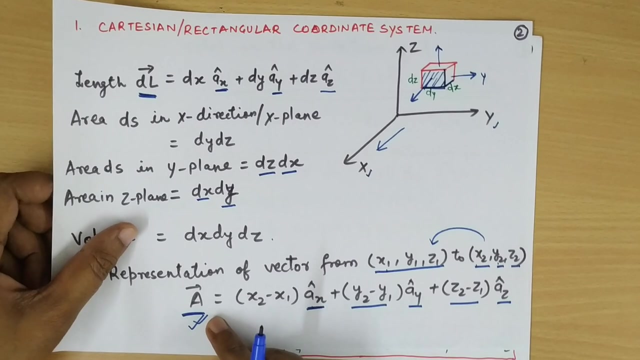 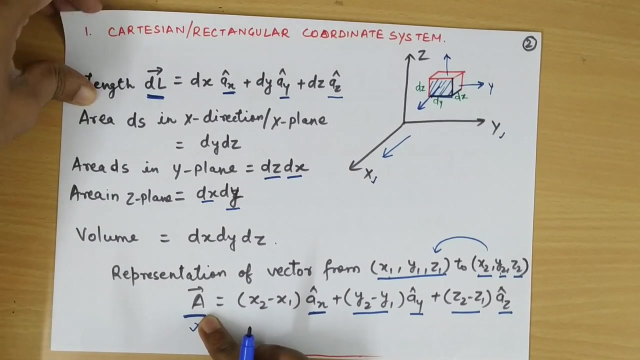 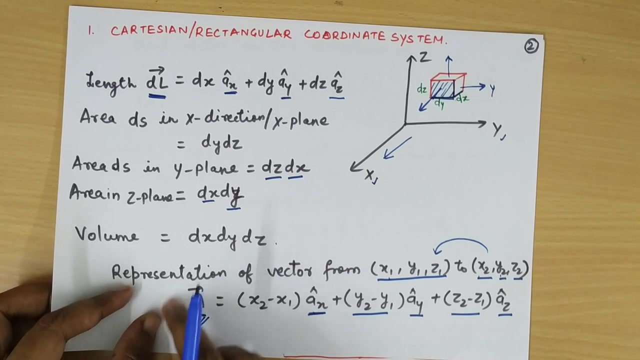 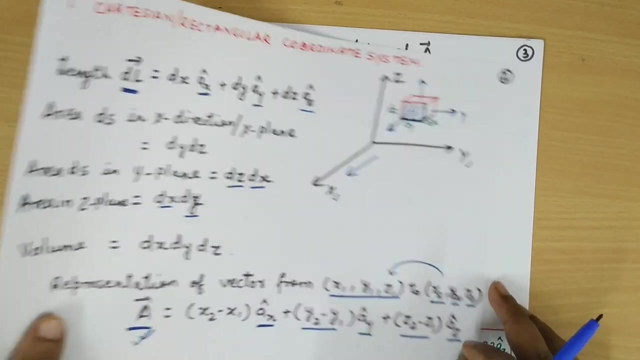 two and write with its unit vector. So vector can be written as: x2 minus x1, ax. ax is unit vector along x direction, y2 minus y1, ay and z2 minus z1, az. So the part y matrix which is the per nucleus. of the unit vectorEv3. The, such as p and z. So the unit vector along this direction can be calculated by dividing this vector with its magnitude. In fact, in any of the coordinate system we find unit vector by calculating its magnitude and dividing it with that magnitude. 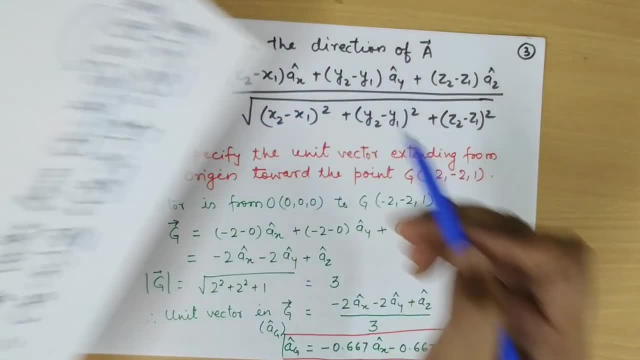 We can calculate the unit vector of that particular vector. So to calculate unit vector we have to find the magnitude of the unit vector that is opened up as describe this options, The of this vector. I have assumed this vector as a, So magnitude of a will be x2 minus x1. 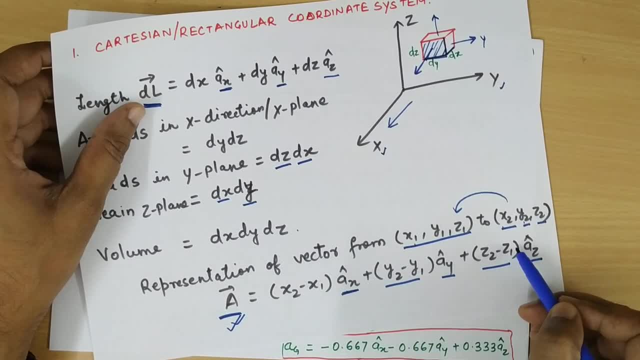 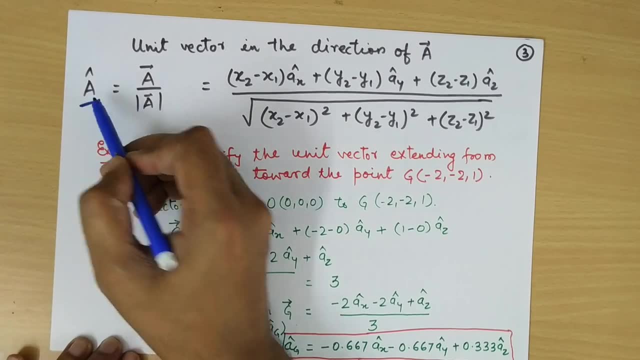 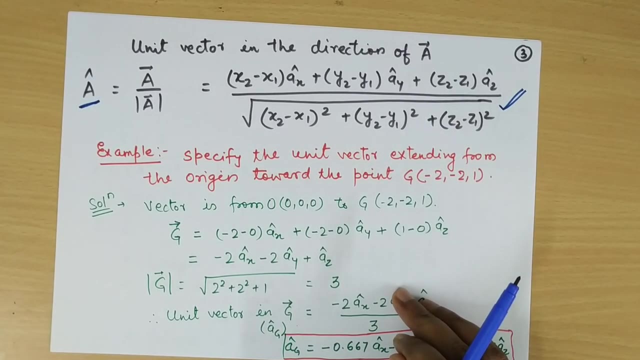 square plus y2 minus y1. square plus z2 minus z1, square square root of 4.. So this is what I have written here. So this is called unit vector, and unit vector can be calculated by dividing its magnitude. Let us take an example. Here we have to specify the unit vector which. 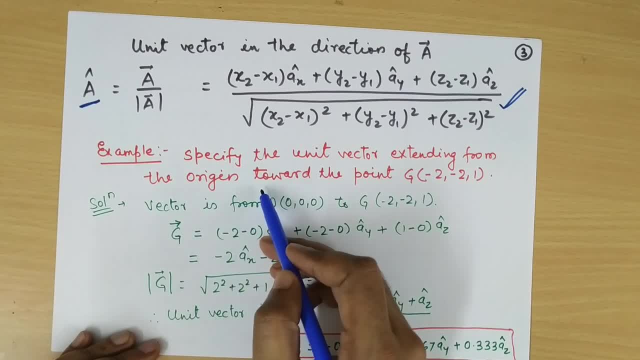 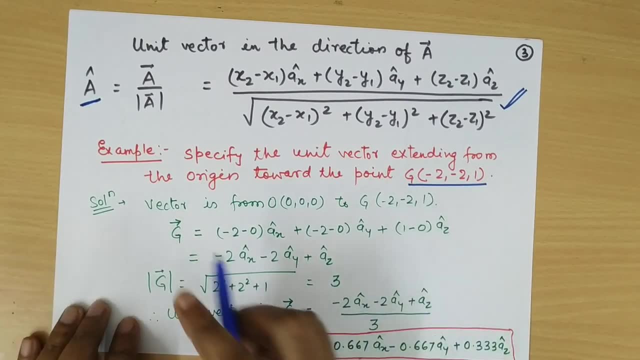 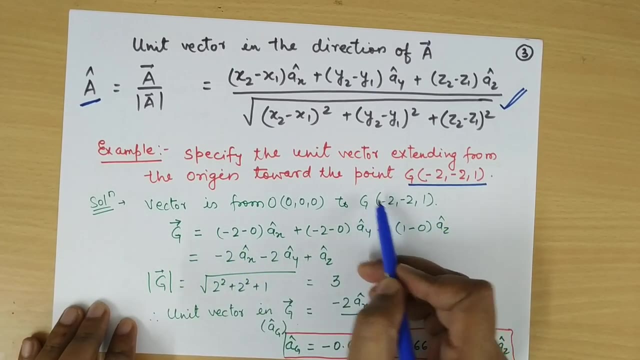 a unit vector of the vector extending from the origin towards the point g, minus 2 minus 2, 1.. So the vector which is extending from 0, 0, 0 to minus 2 minus 2, 1 will be given as the difference of these two points. So in x direction we have minus 2. 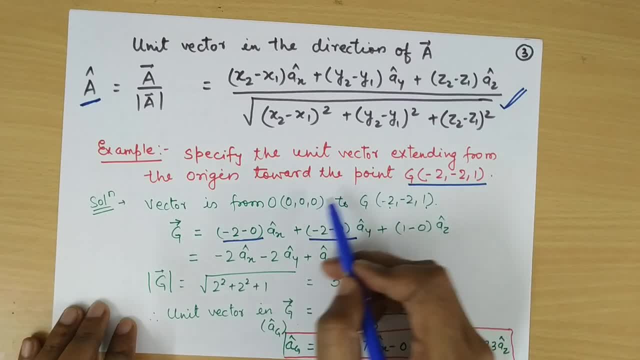 minus 2 minus 2.. So we have a vector which is extending from 0: 0- 0 to x direction, So in x minus 0, y direction minus 2 minus 0 and z direction 1 minus 0. So we will get a vector. 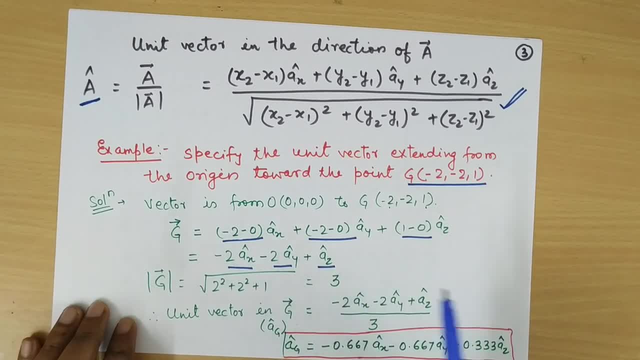 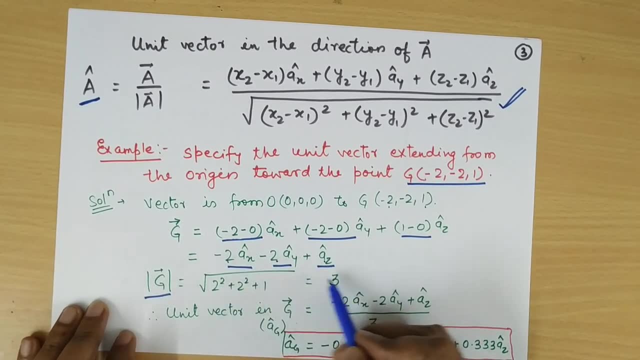 g equal to minus 2ax, minus 2ay plus az, And the magnitude of this vector is 2 square plus 2 square plus 1 square and square root, which is root 9 and equal to 3.. So the unit vector in g will be: 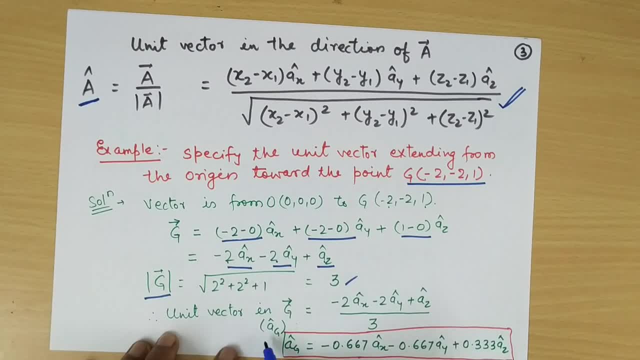 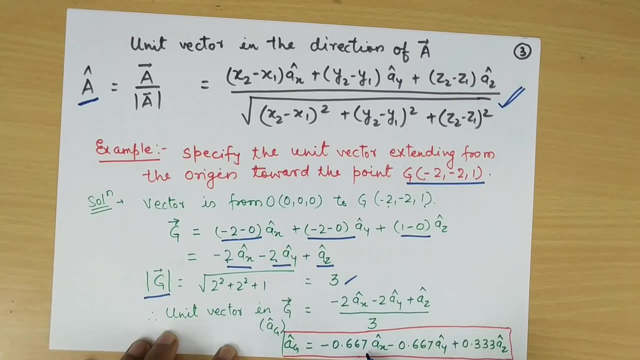 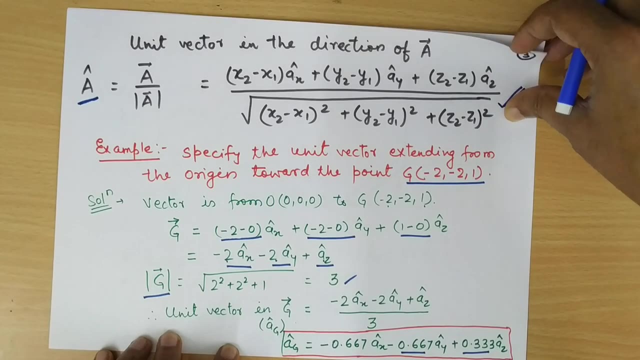 the vector divided by 3.. So the unit vector ag is given by just. if we divide it, we will get minus 0.667, here minus 0.667 and plus 0.333.. So this is how we can calculate unit vector in. 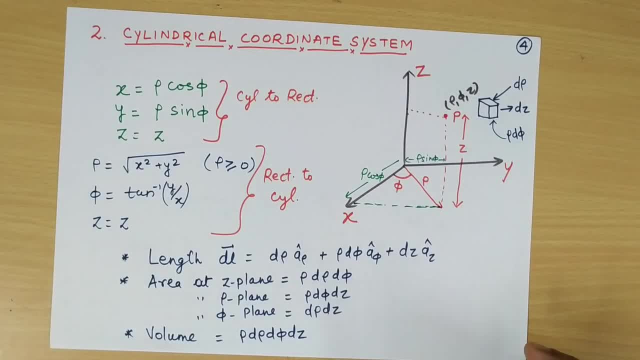 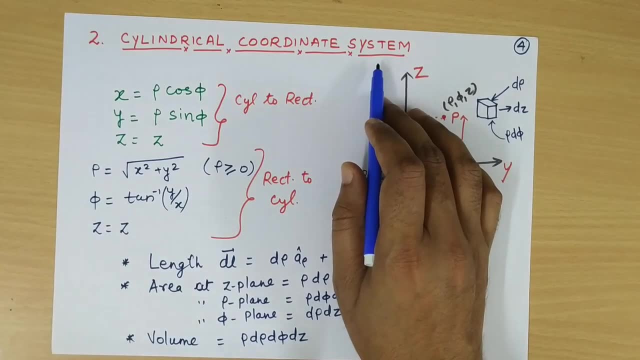 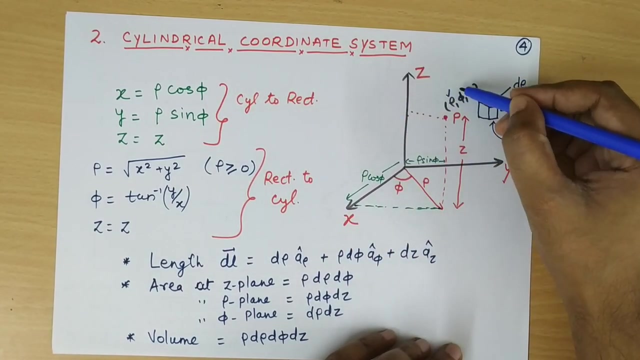 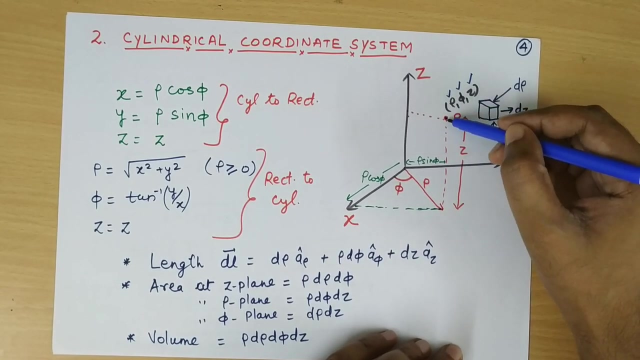 rectangular coordinate system. Now, the second type of coordinate system is cylindrical coordinate system And, as I have defined earlier, in this there are three things: rho, phi and z, where rho is. if this point is defined as rho, phi and z, then we can take the projection of this point on xy. 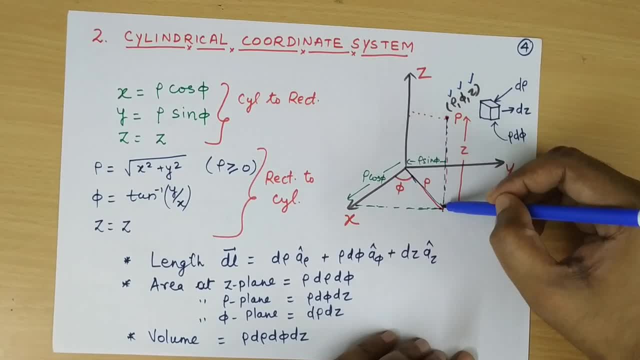 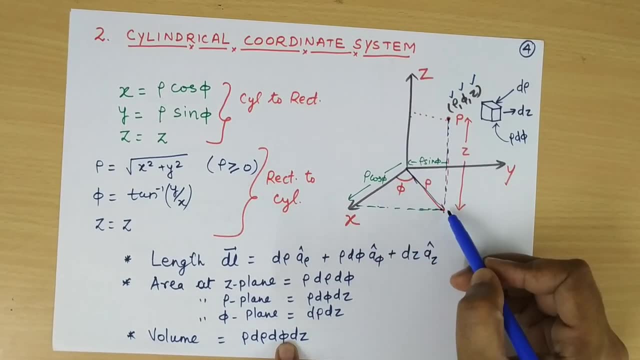 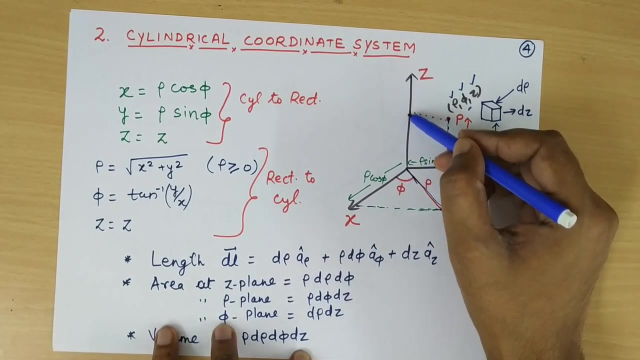 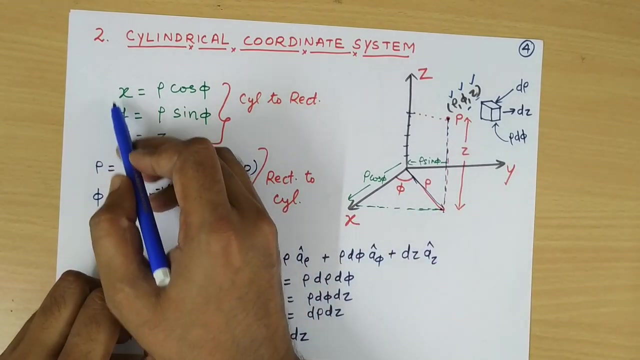 plane and then draw a line, So this length is rho. Then the angle made by this line on x axis is called phi, And z is the number of units in z direction, So it is z. So from here we can find the relation of cylindrical and rectangular coordinate system. 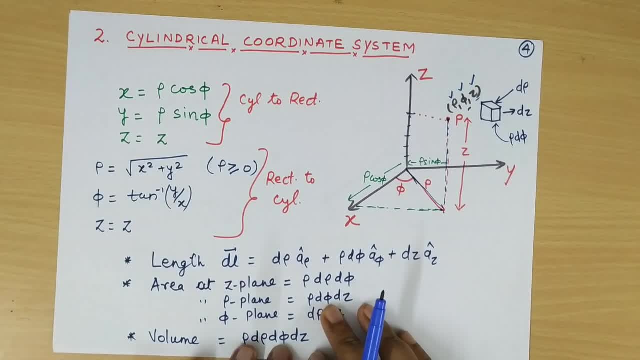 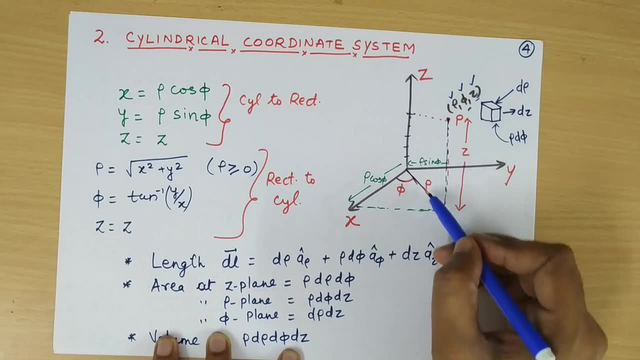 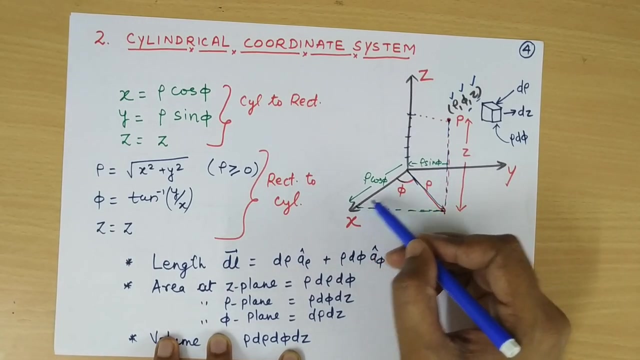 and we can convert the points from one coordinate system to another coordinate system. So here it is rho and phi. So if I take the component in x direction, this will become rho cos phi, because phi is angle at x axis and in y axis it will become rho sin phi. 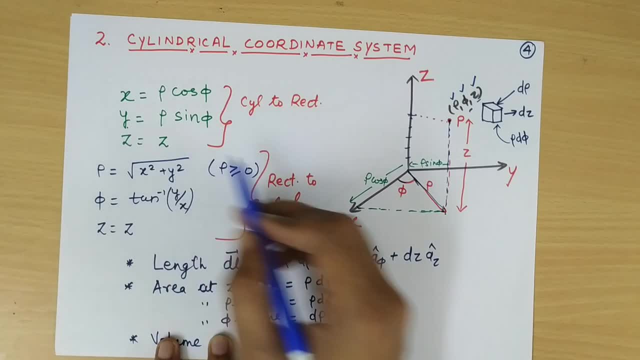 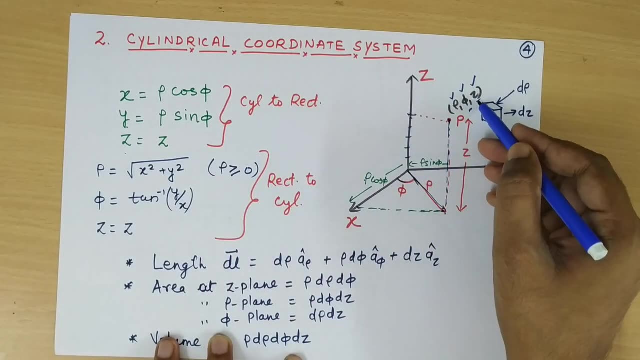 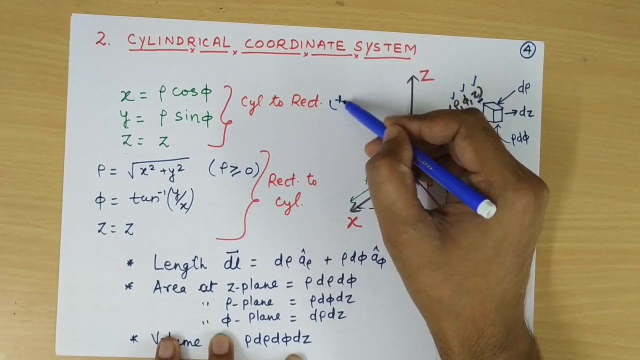 So x is equal to rho cos phi, y equal to rho sin phi and z equal to z, which cannot be changed because z is still there in the coordinate system. So there is one coordinate which is common from the rectangular coordinate system is: 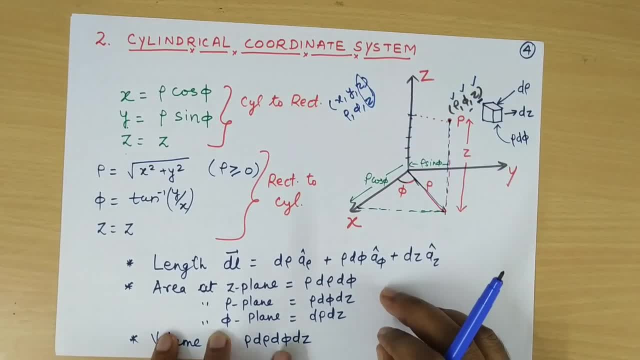 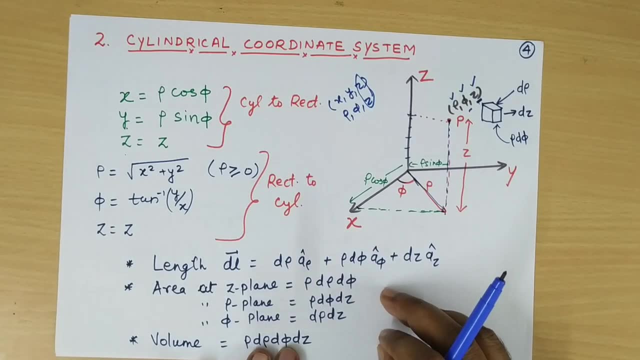 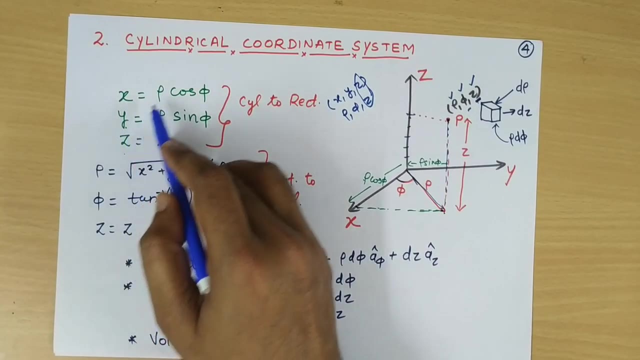 z. This is common, only xy and rho. phi is getting changed. Now when we want to convert from rectangular to cylindrical coordinate system, then we can take a square of these two and add it, So x square plus y square equal to rho. 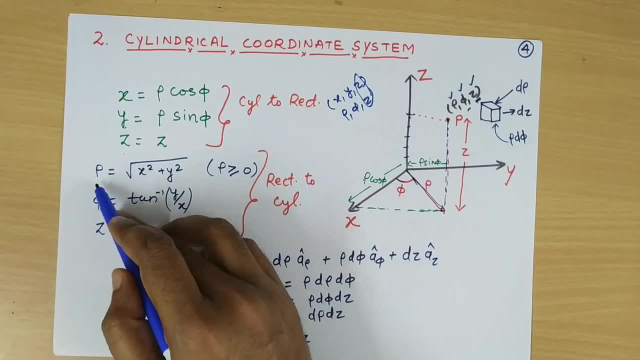 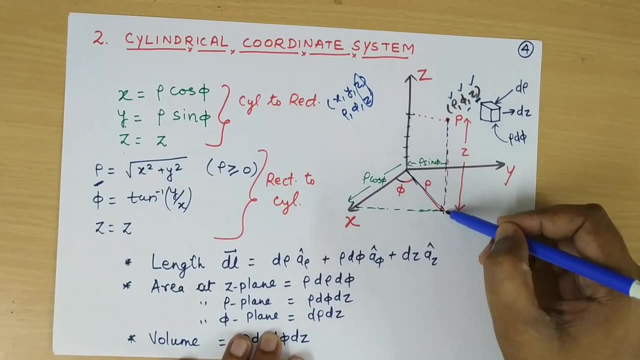 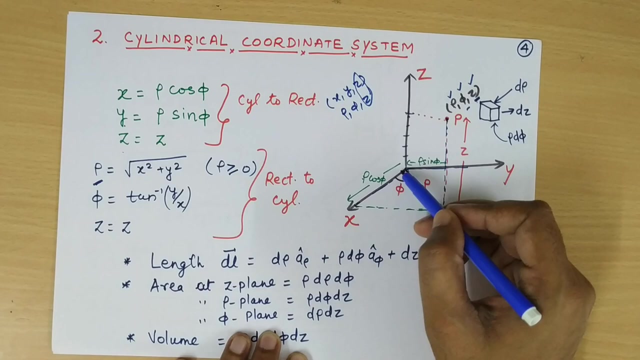 square cos square phi, rho square sin square phi, And we can calculate that rho is under root x square plus y square. Also, from here, this rho is nothing but the root of x square plus y square and the square root of this. So if we calculate x a square plus, 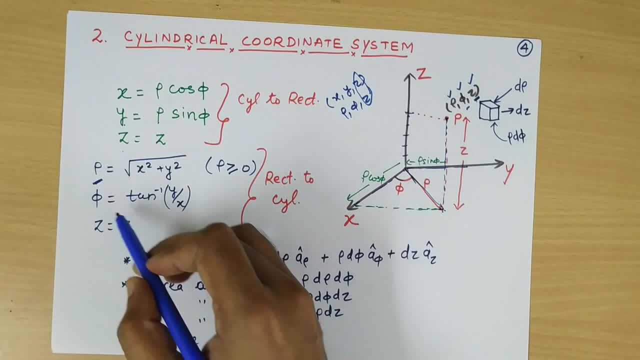 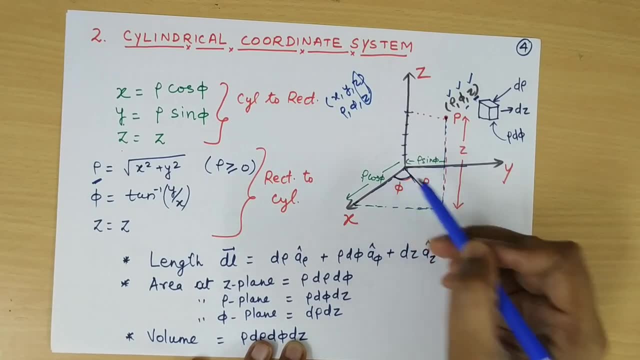 y square square root, we can get rho. Phi is x inverse y by x. So phi is if we take the 10 theta. So this is phi, this is x and this is y. So when we calculate 10 phi, we will get y by x. 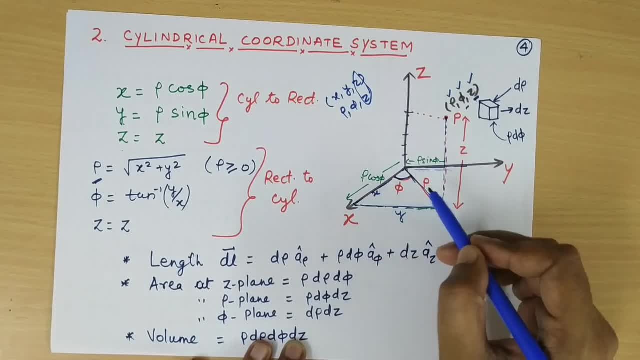 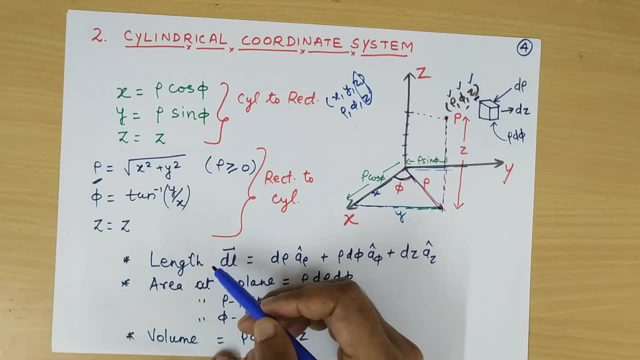 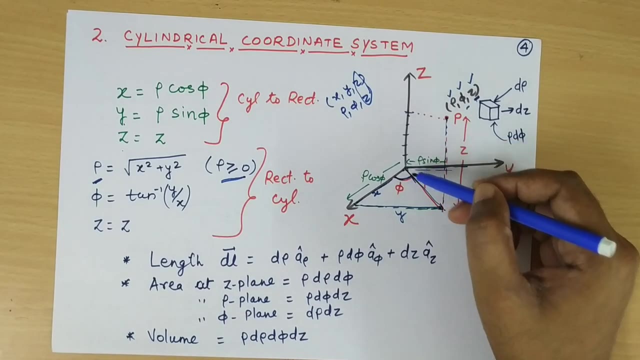 So this is actually y and this is x. so from here we can calculate 10 phi as y by x and z is remain same z. Here rho will be always positive because we are taking the distance from the origin of this projection, which cannot be negative. 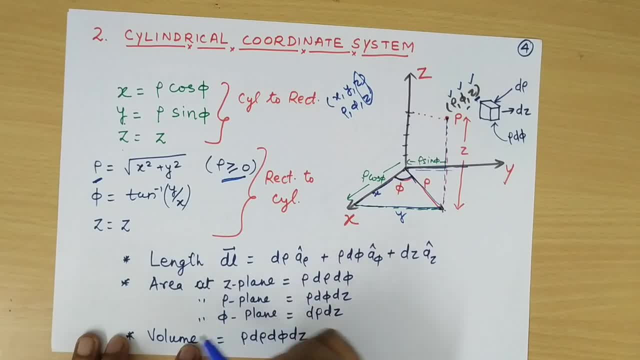 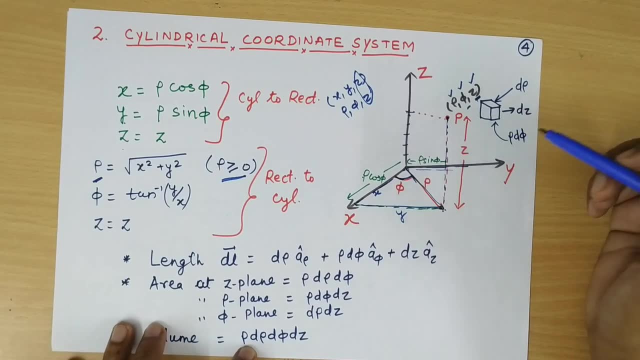 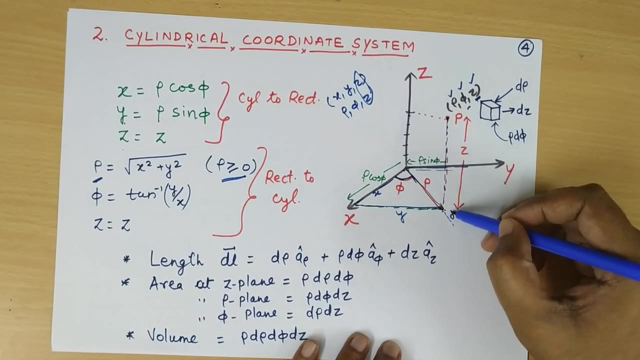 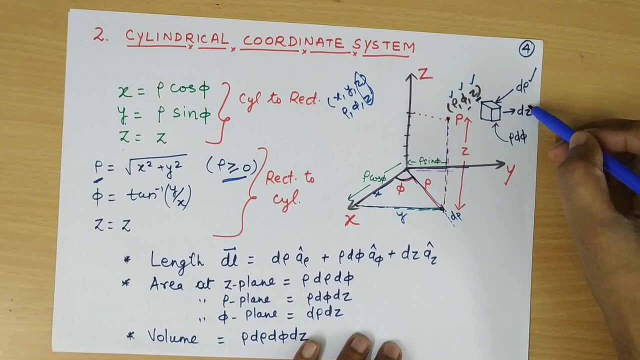 To find length in length, area and volume in cylindrical coordinate system, we have to understand how the incremental length varies. So when we increase length in the direction of rho, that incremental length will be d, rho, which is represented here. If we increase length in z direction, it will be dz, which is represented here. but when we increase length in the direction of 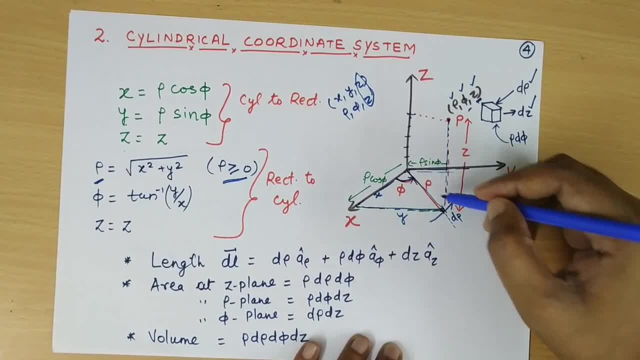 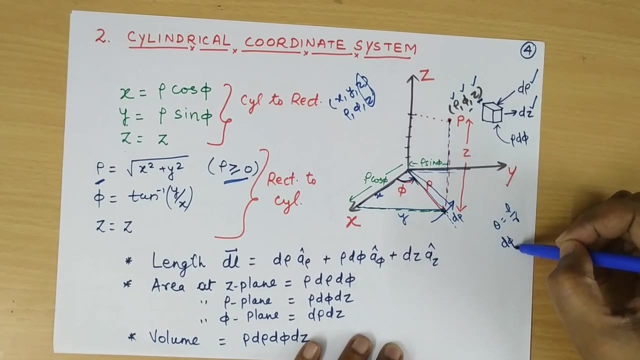 phi. this is the direction of phi. So in that case the incremental length can be calculated as the formula of the arc, which is θ equal to L by r. So here the incremental length is d, phi and there is increase. let's say the arc length is L divided by r. r is rho, So the arc length will be. 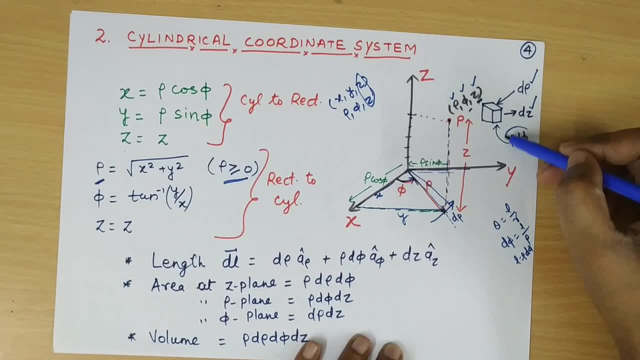 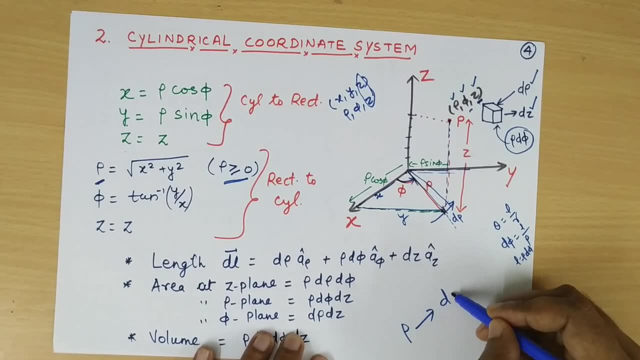 rho d phi. that is why the incremental length in phi direction will be rho d phi. So we can say that the incremental length will be d phi and the incremental length in z direction will be rho d phi. that in rho direction variation is d rho. in phi direction it is rho d phi and in z direction. 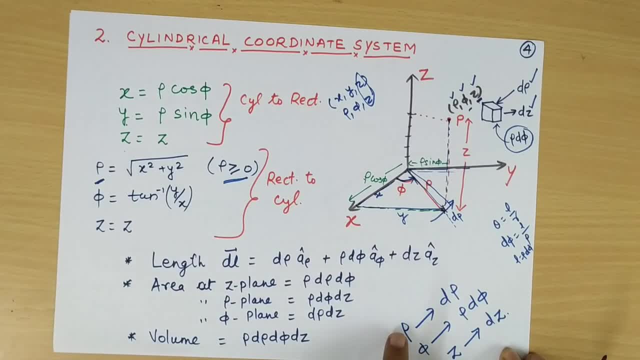 it is dz. So whenever we have any angle in our coordinate system we have to convert that angle into the length. If it is already length, then we can just increase that length. So z and rho, these two are length, but phi is angle. So to convert this angle into length. 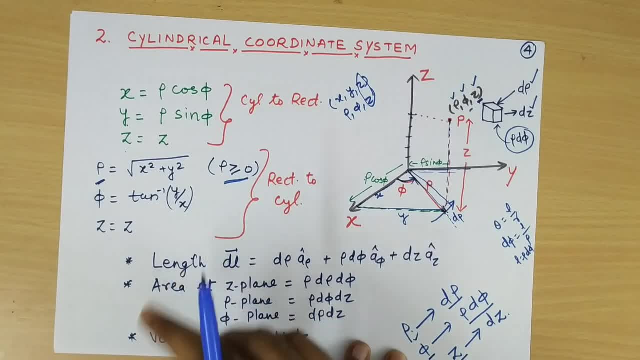 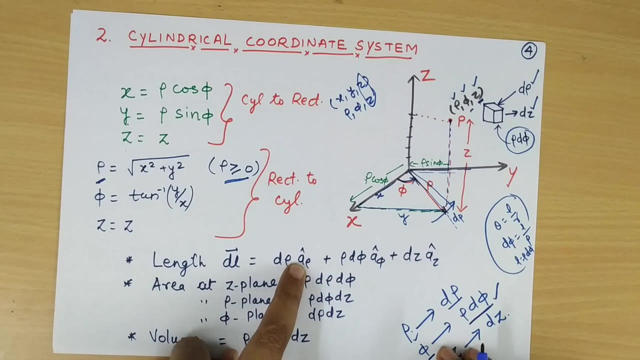 so that we can calculate area volume and length, we have to apply this theta equal to l by r and we can get the incremental length in the direction of phi. So length dL will be d rho a rho A rho is unit vector in rho direction. Rho d phi a phi in phi direction. 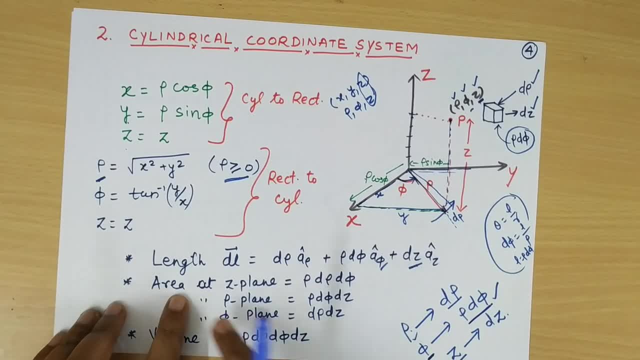 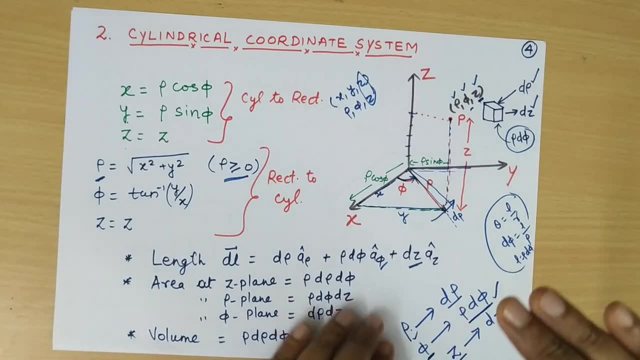 And dz lambda sorryantes, z in z direction. Similarly, area at z plane. z plane means the top plane of the cylinder. When we have a cylinder on top plane, we have. that is called z plane. So area in z plane will be. 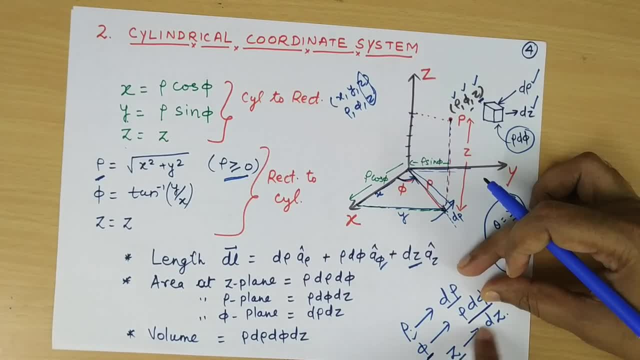 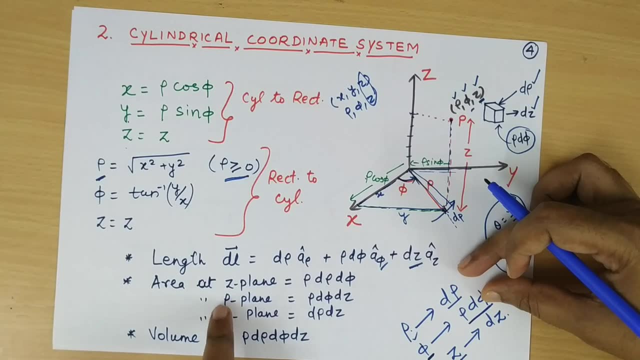 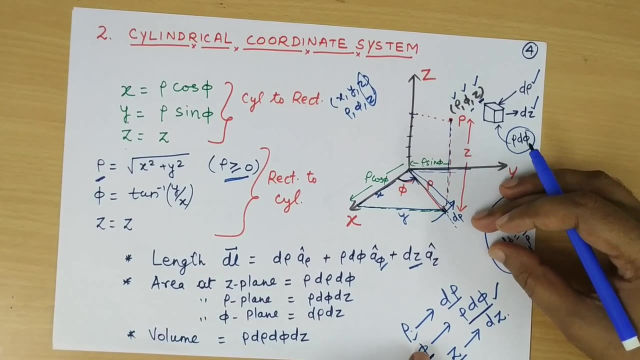 multiplication of these two. When we are finding area over here on z plane, we have to multiply these two. we will get rho d rho d phi, So rho d rho d phi When we are calculating area at rho plane, rho plane means the curved plane of the cylinder In that plane. since we are finding at 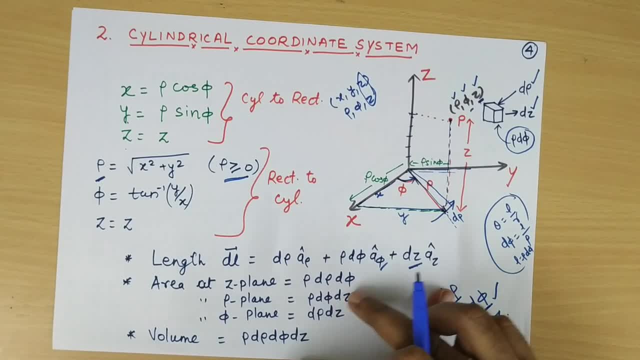 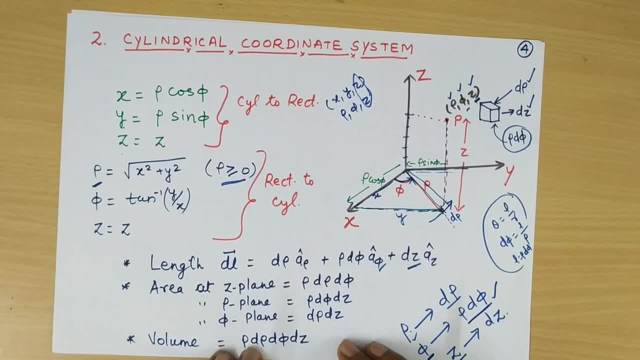 rho plane. so we have to multiply rho d phi d z, So it is rho d phi d z. Now in third case, when we are calculating area at phi plane, so it will become d rho into d z, which is again. 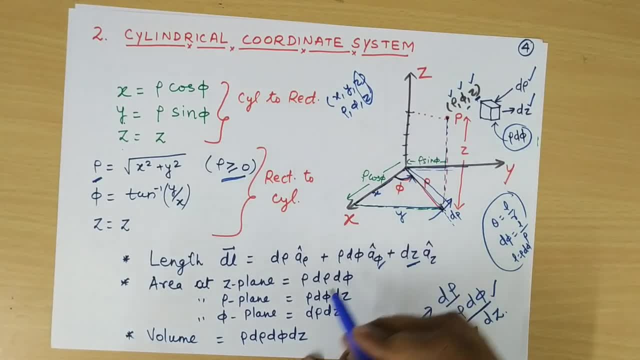 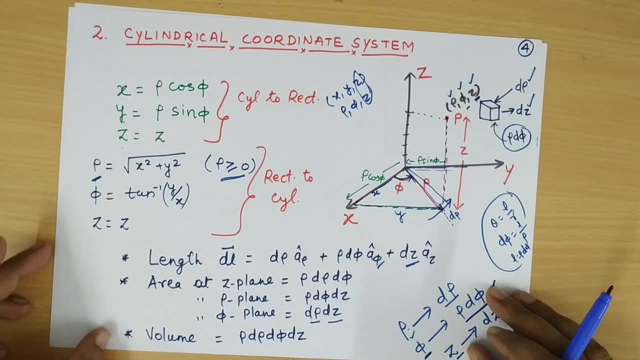 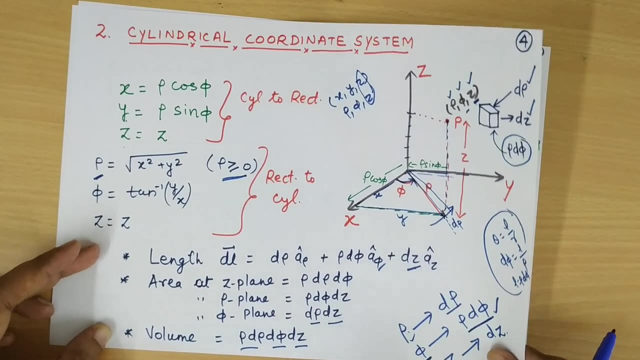 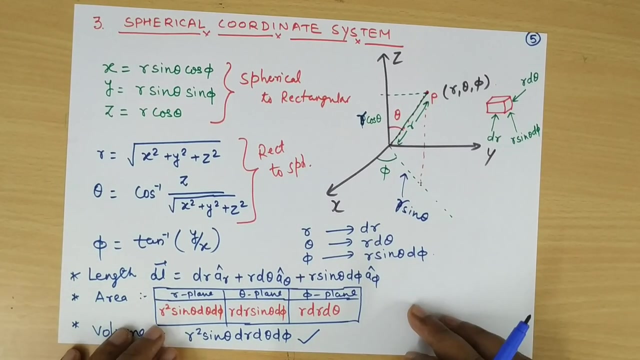 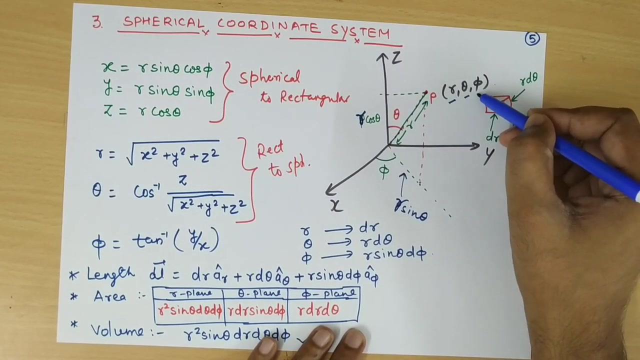 area on the phi plane. So we can multiply d, rho and d z to calculate that. So the total volume will be rho, d, rho, d phi and into d z. The third type of coordinate system is a spherical coordinate system, And here we have three coordinates, known as r, theta and phi. So these two coordinates are equal to 0. So if you find a 0, then you have to multiply 0. So we can multiply d rho and d z to calculate that. So the total volume will be rho d rho d phi and. 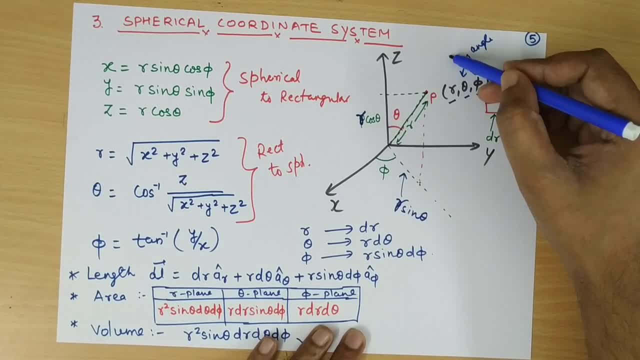 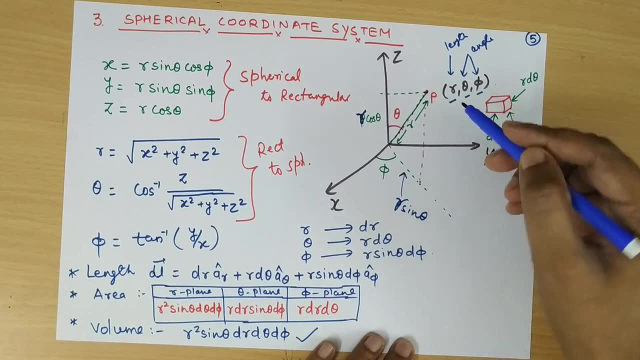 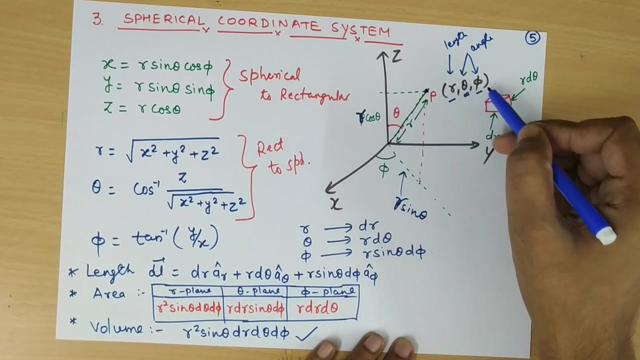 2. theta and phi is angle and r is length. So to calculate r, r is the distance from origin to the point, So this is r. Theta is angle, made on z axis, So that is theta and phi is same as the cylindrical coordinate system means the projection of this point over. 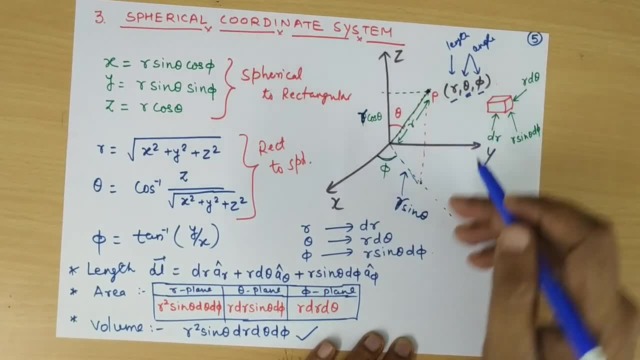 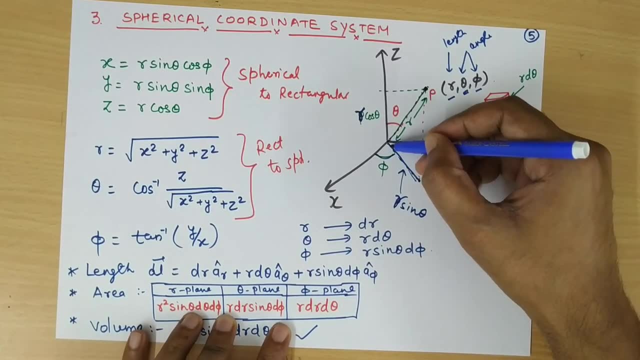 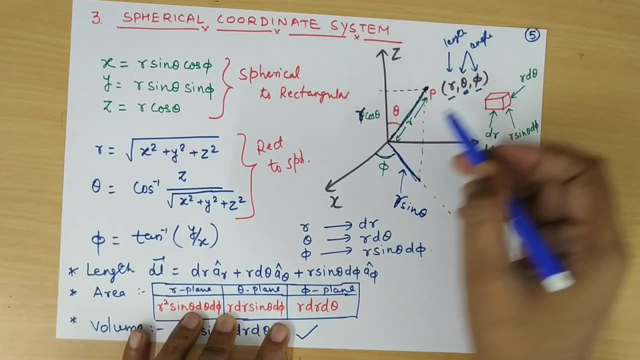 x, y plane and then angle made by x axis is phi. So to calculate x, first of all we have to calculate this, because here rho is not defined, rather r is defined. So when we take r here and angle is theta, so this length will become r cos theta and 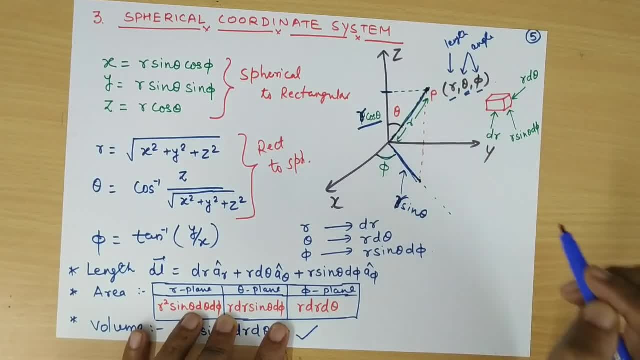 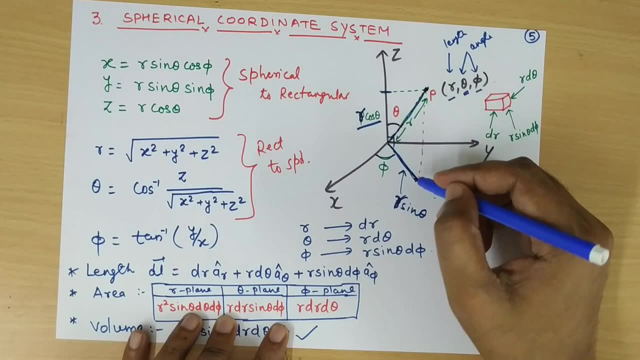 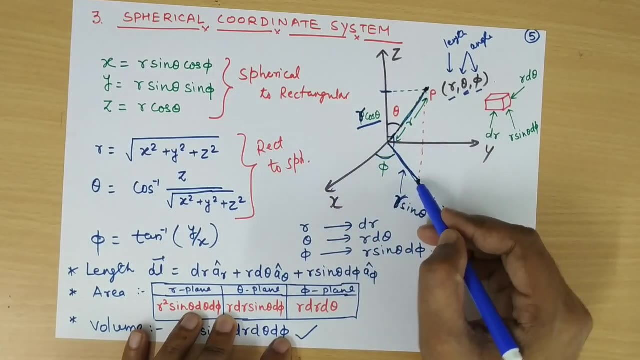 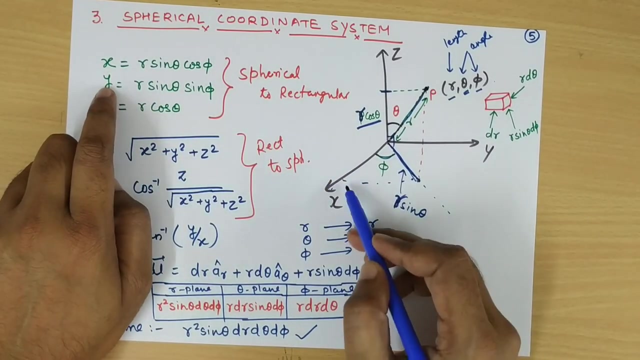 its projection length will become r sin theta, So projection is on x y plane means this is actually 90 degree. So projection will be r sin theta So r sin theta. So x is equal to r sin theta into cos phi. So this will become x and y is r sin theta sin phi, So r sin theta sin phi. 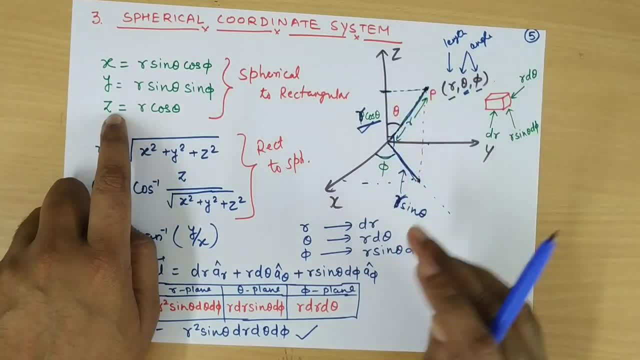 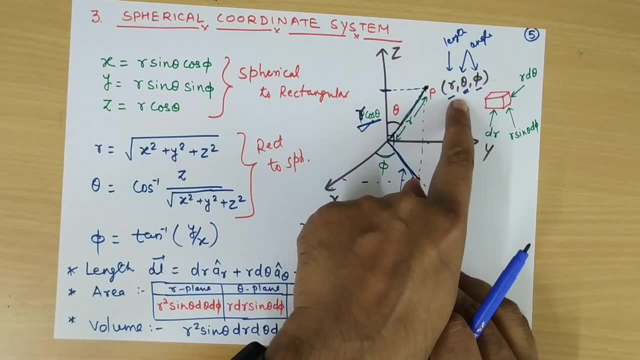 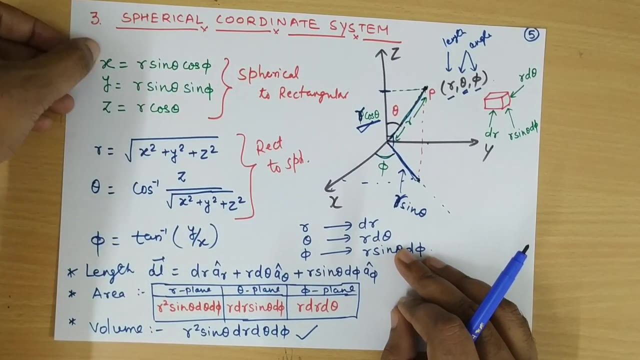 and z is equal to r cos theta, which we have found from here. So this is how we can convert any point given in a spherical coordinate system as r theta phi. We can put the value of r theta phi to find its corresponding rectangular coordinates or rectangular coordinates points And vice. 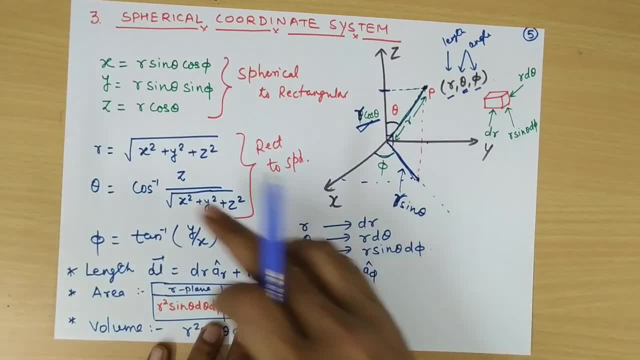 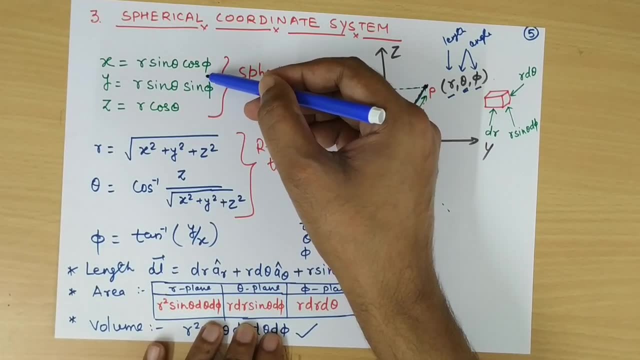 versa. we can also calculate r, theta phi by knowing x, y and z. So r will be x square plus y square plus z square, Which can be easily converted from here, And theta is cos inverse. From here, we can say: 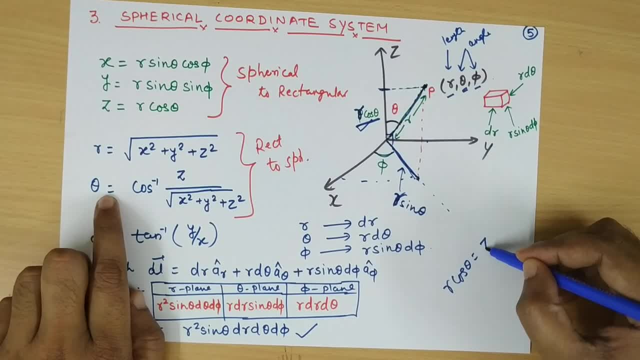 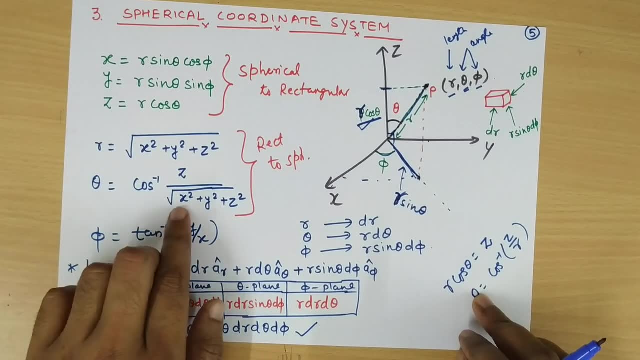 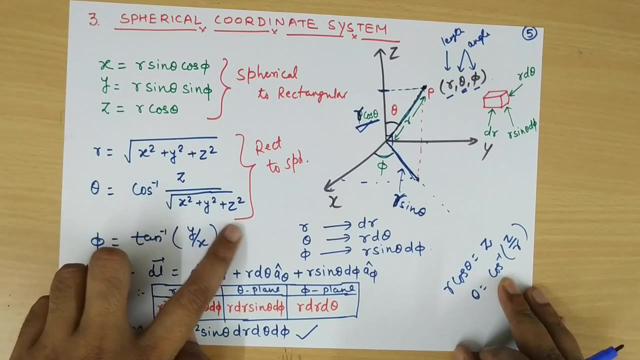 r cos theta equal to z. So theta will be cos inverse z by r, And r is under root x square plus y square plus z square. So theta is cos inverse z by under root x square plus y square plus z square, And phi is same as the previous one in cylindrical coordinate. 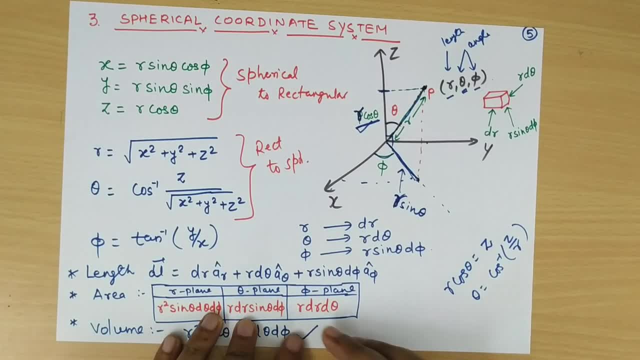 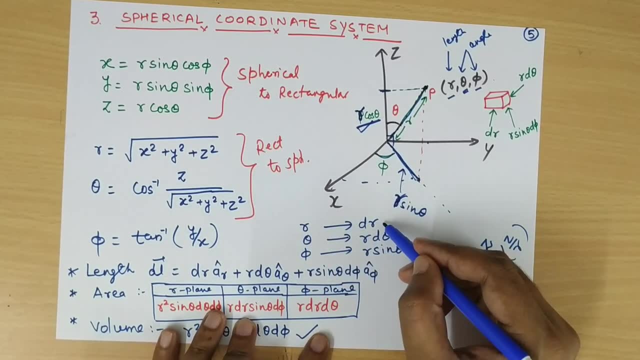 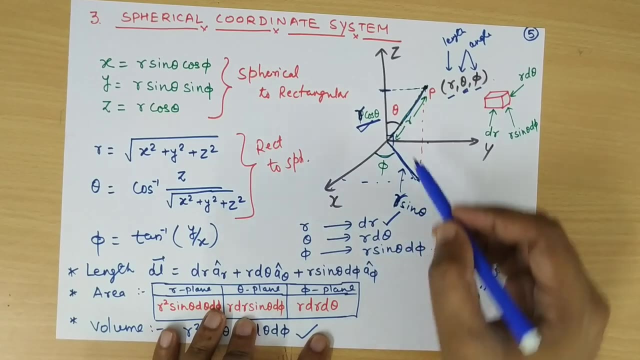 system It was tan inverse y by x. Now the variation in different coordinates: in r direction, since it is directly length, So it will be dr. Theta is angle, So in the direction of theta it will become r d theta, as r is the radius of the arc. So in this direction the change. 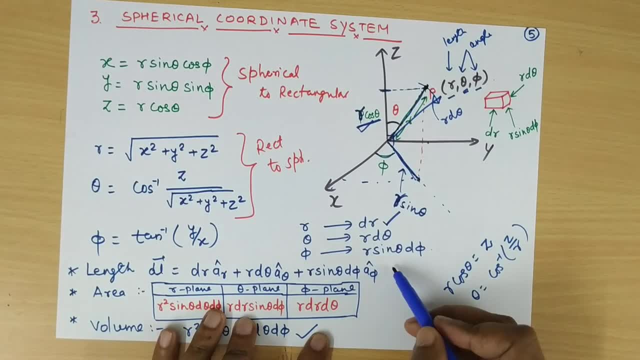 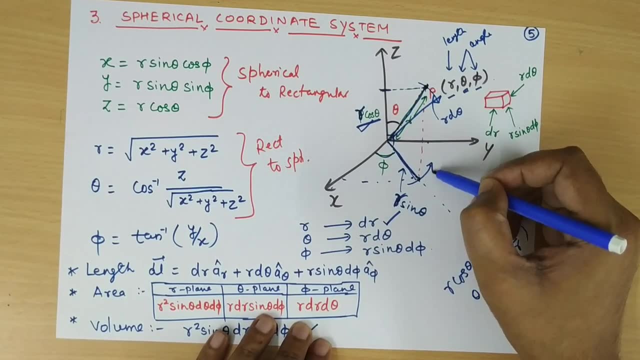 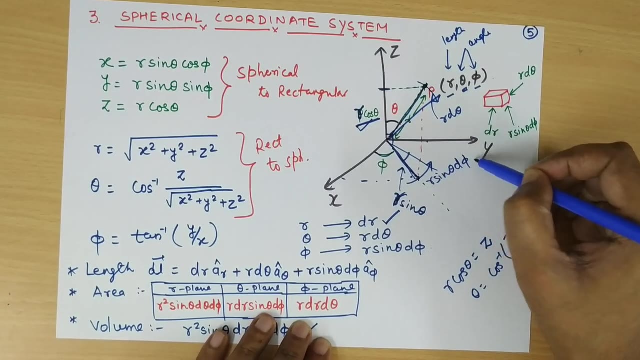 will be r d theta, And in the direction of theta, it will become r d theta. So in this direction of phi, since this is r sin theta, So in the direction of phi, we have r sin theta multiplied by d phi, So this will become r sin theta d phi. So we have found the incremental. 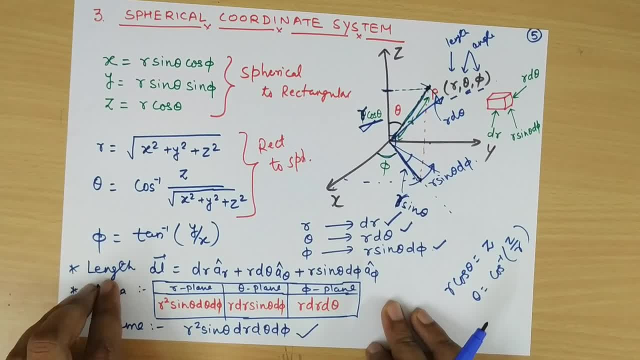 length in all the three directions. Here we can write length as dl, dr, ar, then rd theta, a theta And r sin theta, d phi, a phi And area as d phi at a, A, e, phi. let us give L of c plus r by d phi And a Y, then D, I get basically r, d, each of this half of Half. of S And now they are simple single order. For e, phi we find the r, d, 약간 of r or d rather than a, e and the error So between both families in point types. So if in this 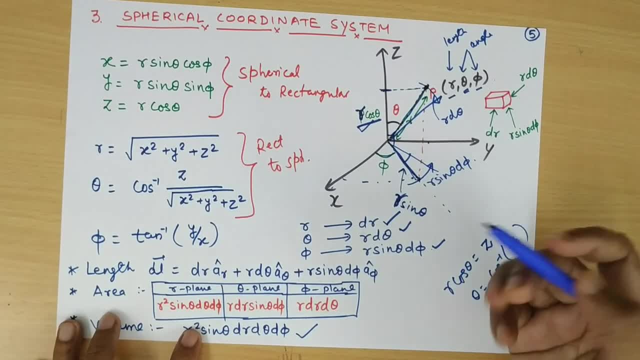 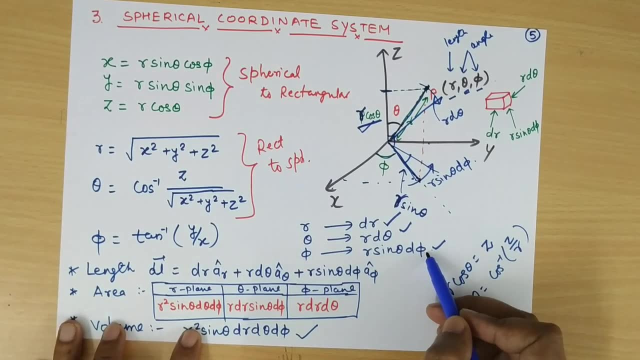 case we predict length B as d we have equal length. hence let's calculate dip judgement area for different plane in r plane. when we are writing in the r plane, then it will become r d theta into r sine theta d phi, which is r square sine theta d theta d phi, the multiplication. 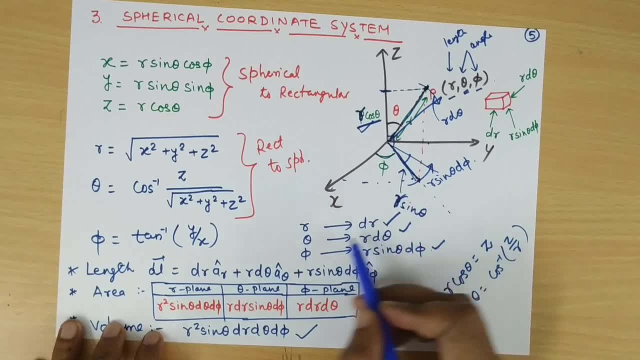 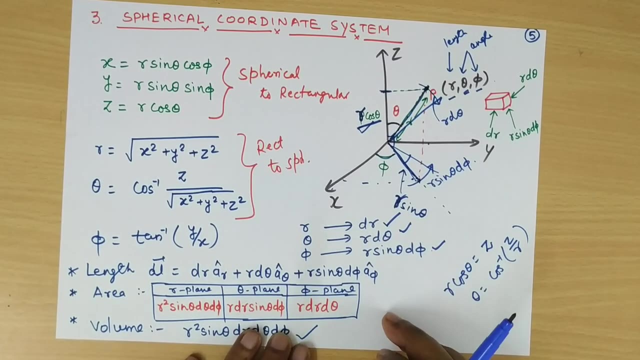 of these two when we are finding for theta, then multiplication of the first one and the third one, so it is r sine theta dr d phi, r sine theta dr d phi. when we are finding for the phi plane, it will become r dr d theta, so it is r dr d theta, and hence we can calculate the volume as r square.